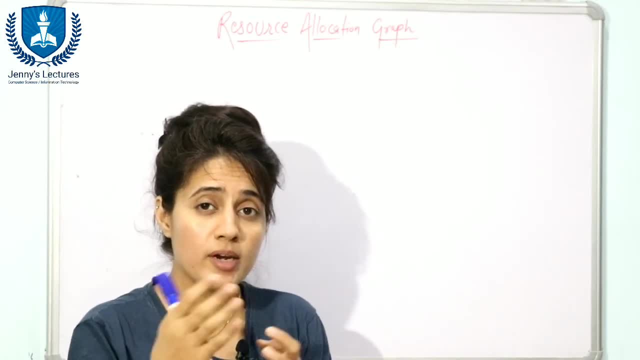 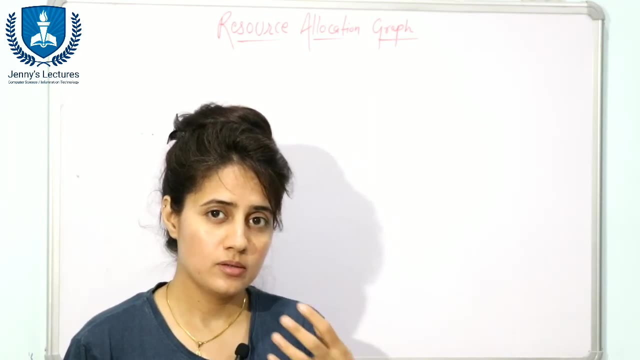 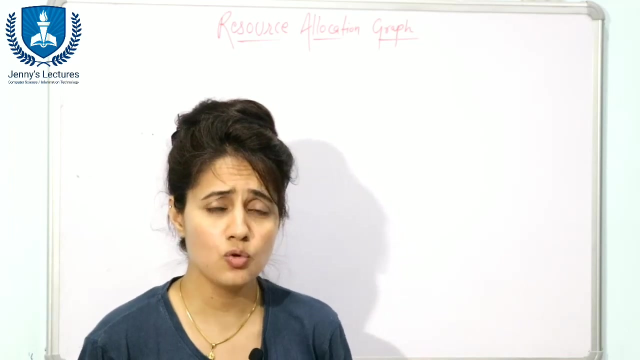 All the type of resource allocation graph: resource allocation graph with one instance of resources, with more than one instance of resources. Plus one more thing: how you can see that there would be a deadlock only by seeing the resource allocation graph. We will also discuss that thing. So what is resource allocation graph? See, if you are taught with the help of some diagrams or graphs or pictorial view, then I guess you get the concept easily. 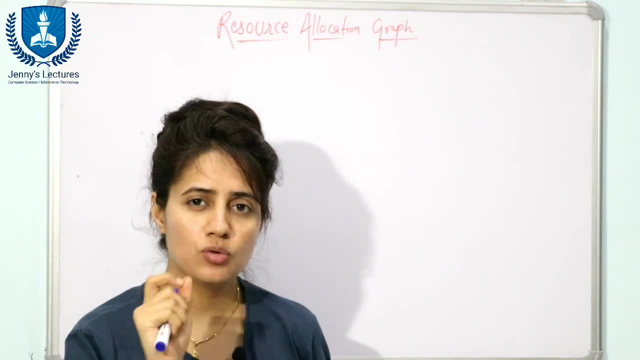 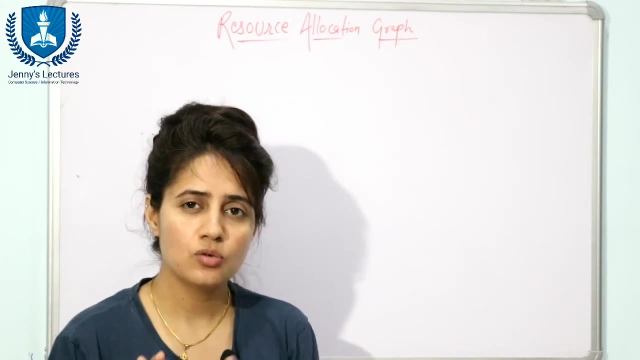 So to describe the deadlock in a better way, or you can say, to describe deadlock more precisely, some directed graphs would be used, and those directed graphs are known as resource allocation graph, or you can say system resource allocation graph. See, as the name suggests, resource allocation graph, how the resources are to be allocated among processes. That thing is represented using graphs and that is known as resource allocation graph. 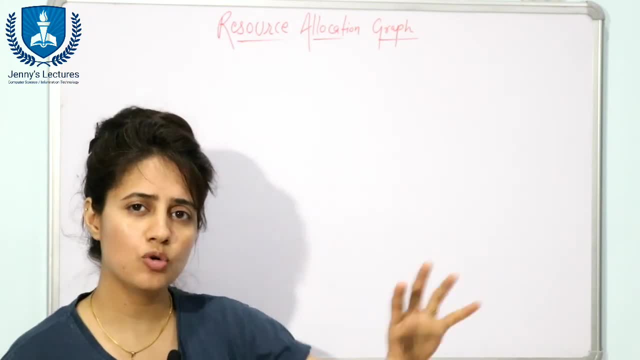 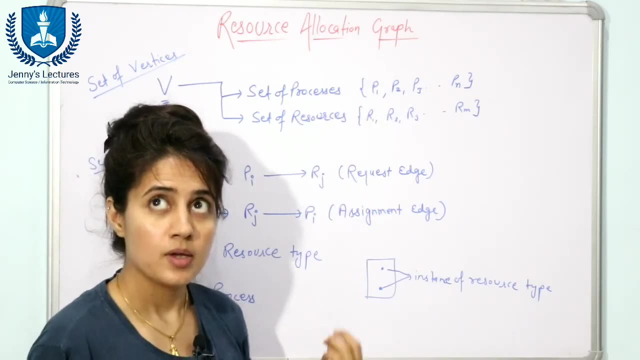 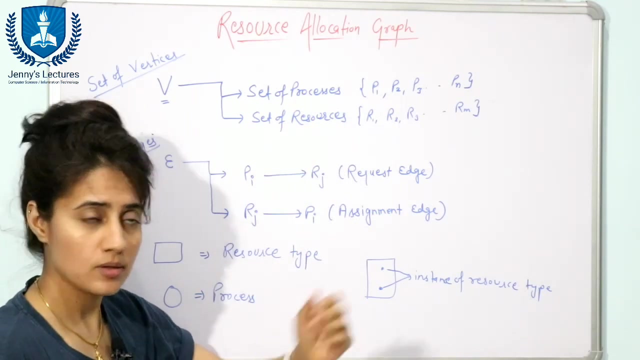 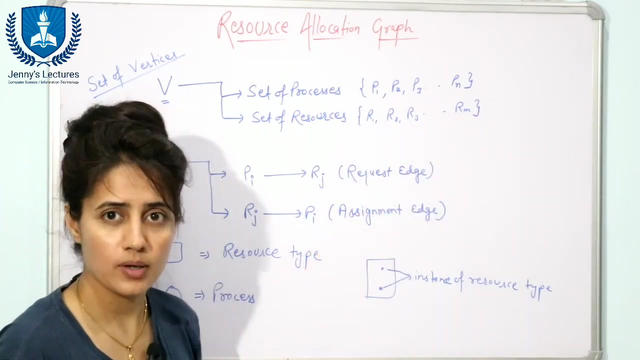 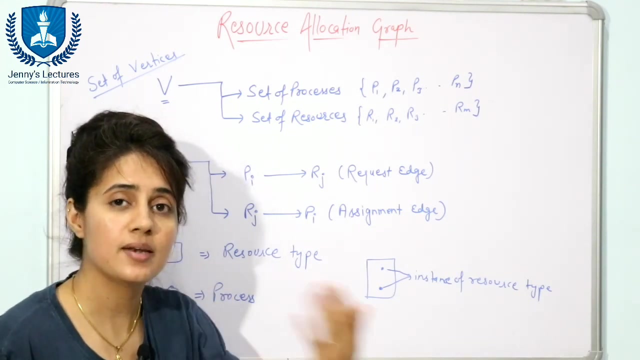 So these are basically used To describe the deadlock more precisely. Now, if we are talking about graph, then obviously there would be set of vertices and set of edges. Okay, Here also we have set of vertices V. Now here we have two type of set of edges. One is set of processes, maybe suppose from P1 to Pn, and next one is set of resources: R1, R2, R3 to Rm. Now, set of edges. Edges are also two types. One is request edge and one is assignment edge. 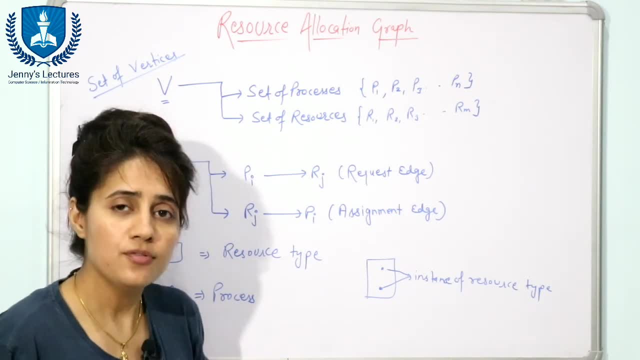 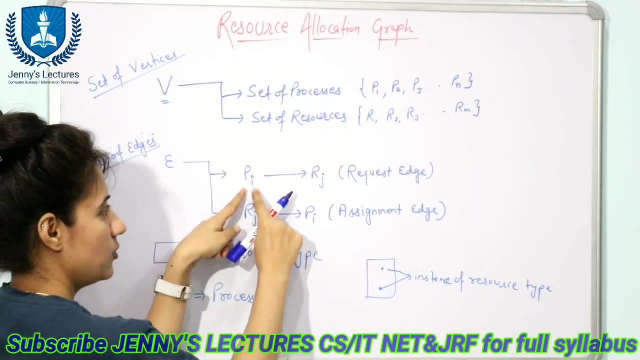 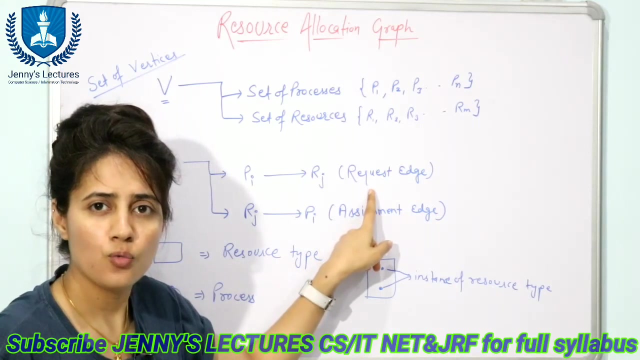 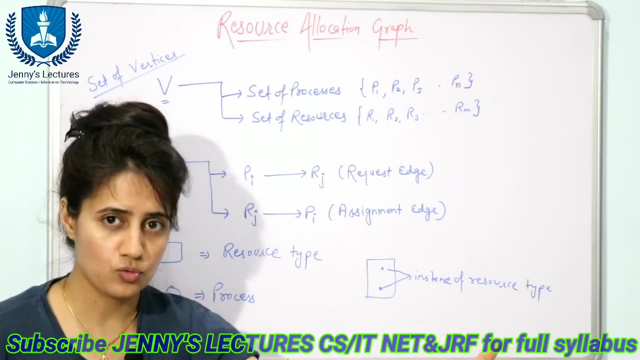 Request means if a directed edge is from process to resource, like this- Suppose process is PI and this direction of this edge is from process to resource, then this is known as request edge. Here you can say a process is requesting for some resource, or you can say and waiting for that resource, And if that resource is available and that resource is, you know, assigned to that resource, then this is known as request edge. 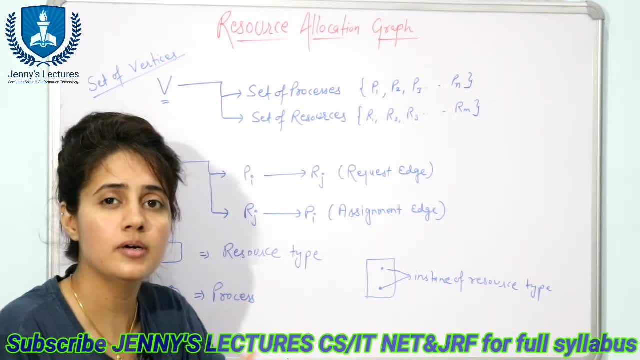 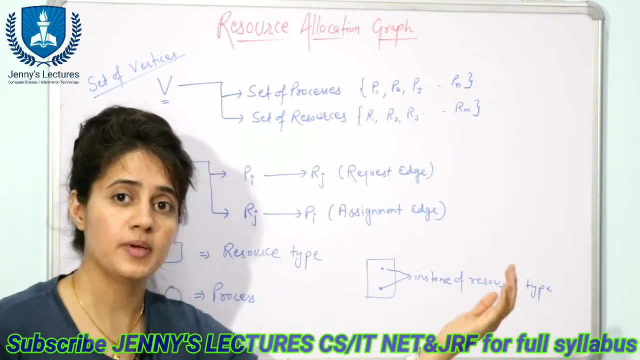 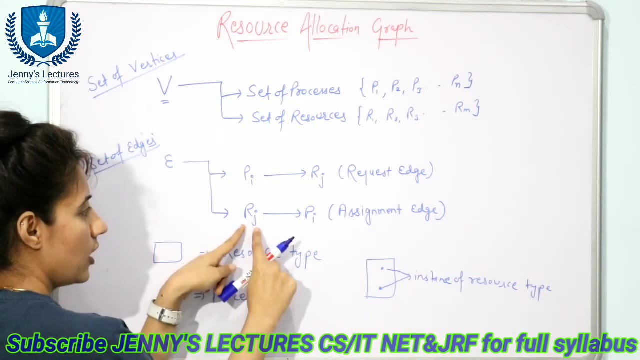 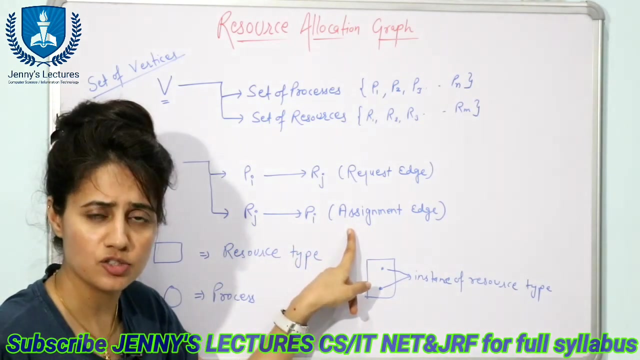 Then this request edge would be turned into assignment edge. Assignment edge and edge would be in opposite direction from the request. edge means it would be from resource direction would be from resource to process, like this: Resource RJ to process. direction would be like this, And this is known as assignment edge means that that resource has been allocated to that process. 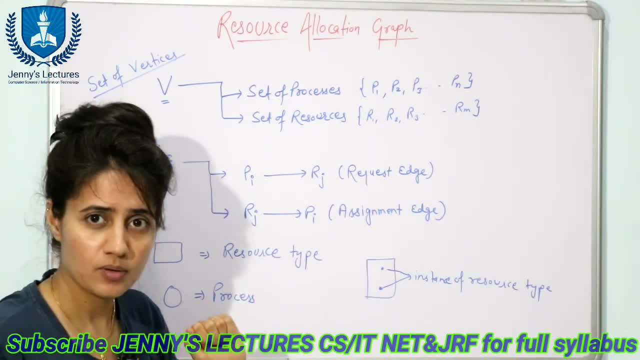 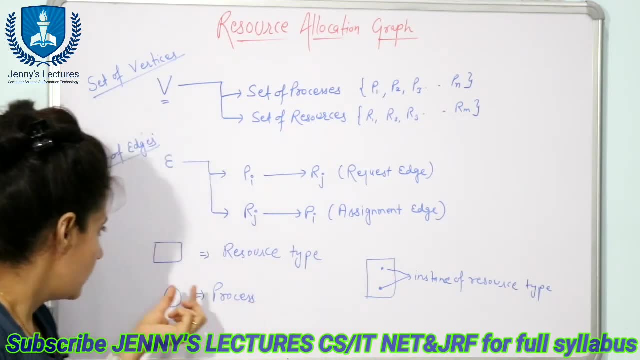 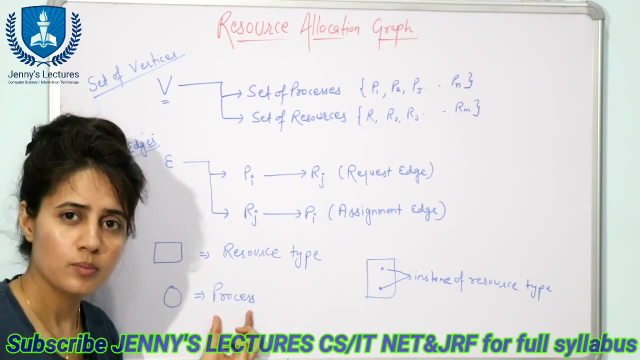 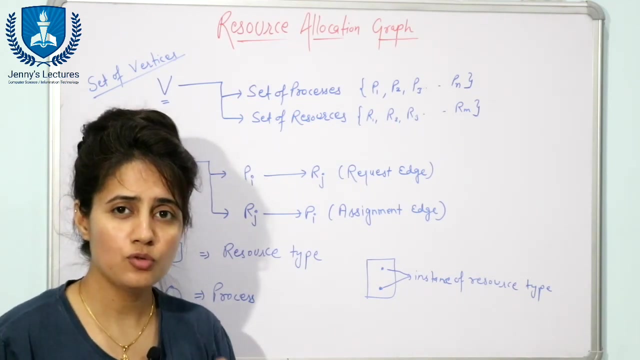 Two types of edges are there: Request and assignment. Fine, Now how to represent that process, how to represent a resource? and like this in this graph, See, this square would be used to represent a resource type. This circle would be used to represent a process. One more thing: What is instance of a resource type, See? instance means, let us suppose we have two processors, Then you can say, or you can say two CPU, Then you can say, we have two. instance of a resource type. 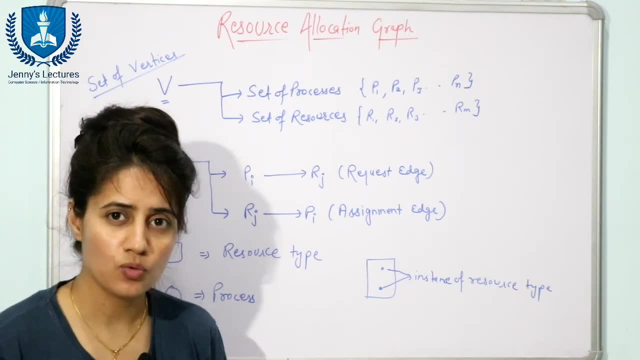 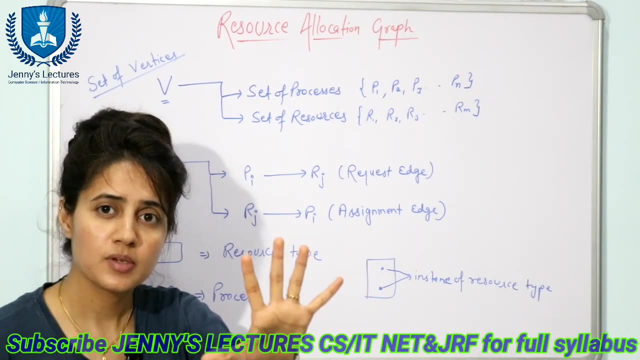 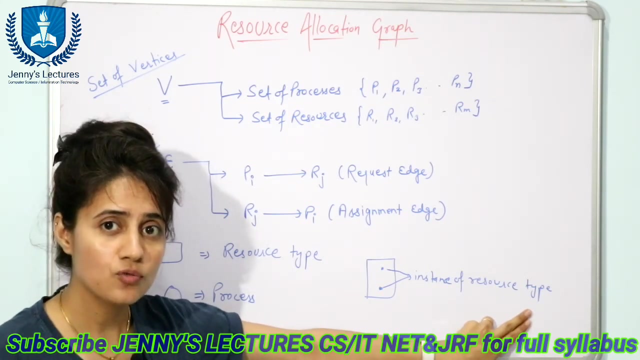 One resource type CPU, or you can say one printer is there. So resource type is what Printer? And if we have five printer, then you can say resource type is printer and instance of that resource is five. We have five instances of a printer or you can say five instances of a resource type printer. So instances would be represented with the help of these dots. 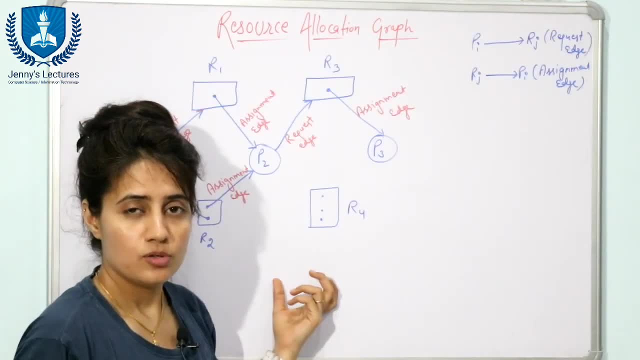 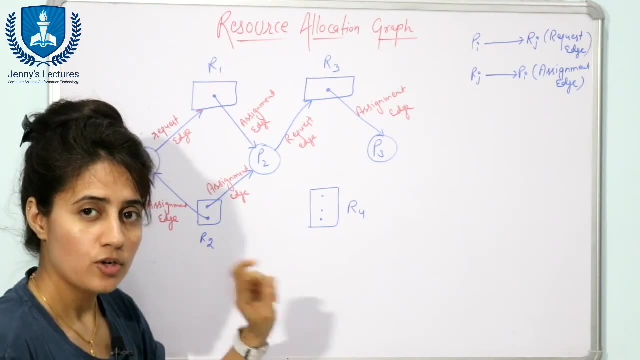 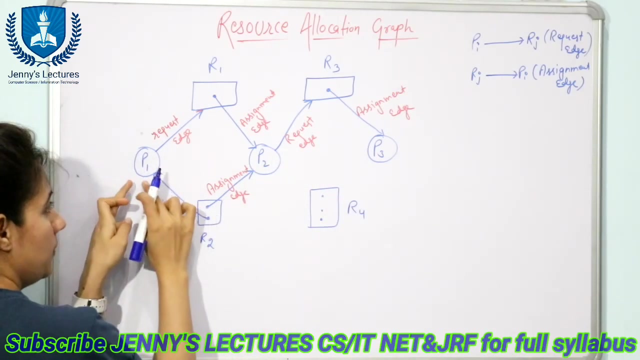 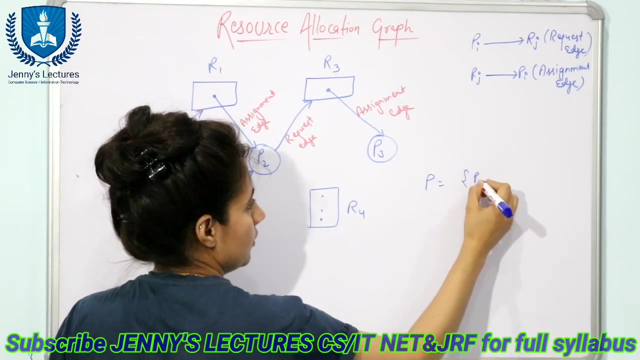 Within this square, or you can say rectangle. Now let us take this resource allocation graph, See. in this case, as you can see, we have set of vertices means we have set of processes and set of resources. So set of vertices are, see: P1, P2, P3. These are set of processes. Fine, You can write like this: P1, P2 and P3.. 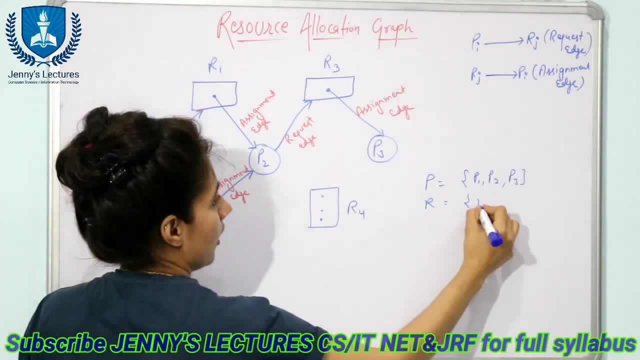 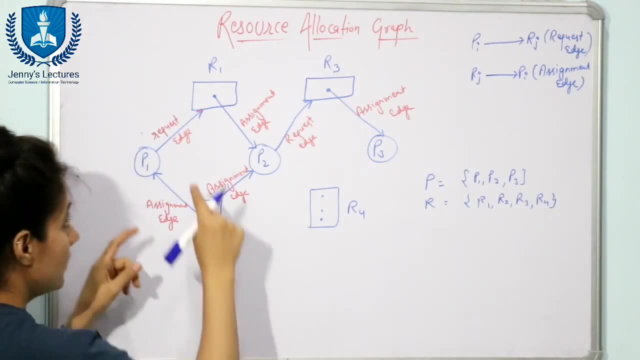 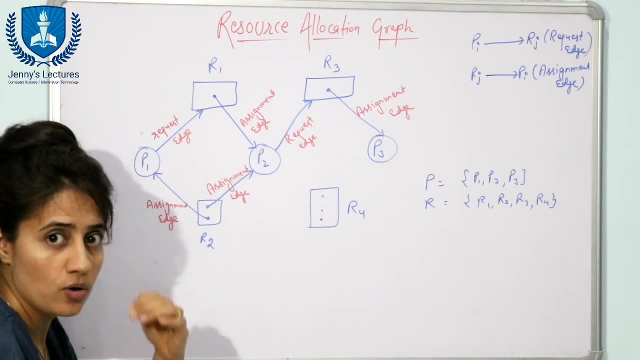 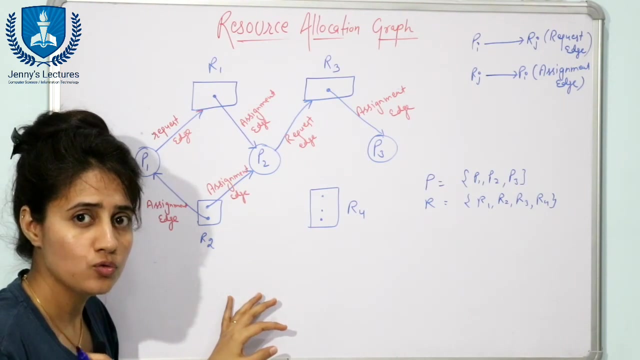 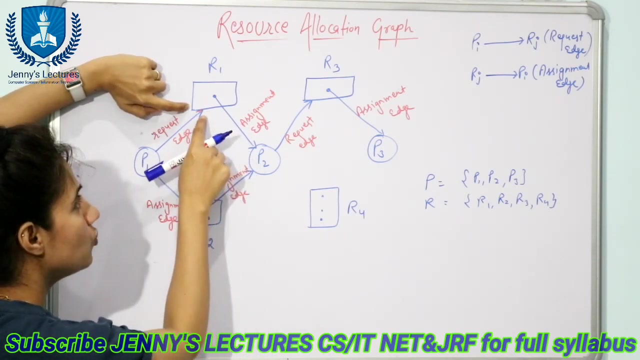 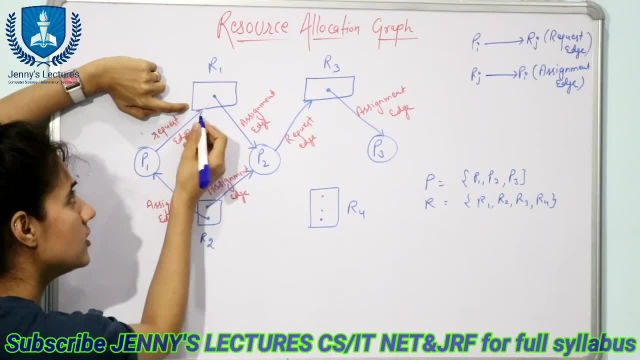 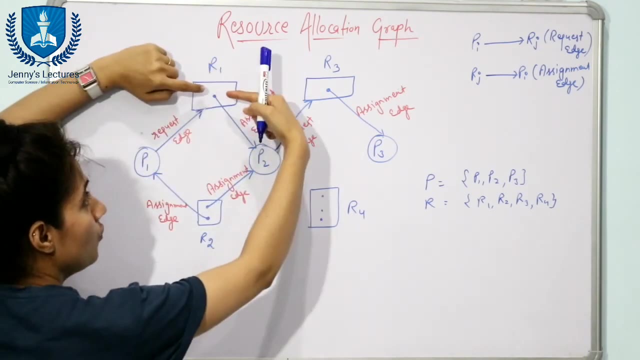 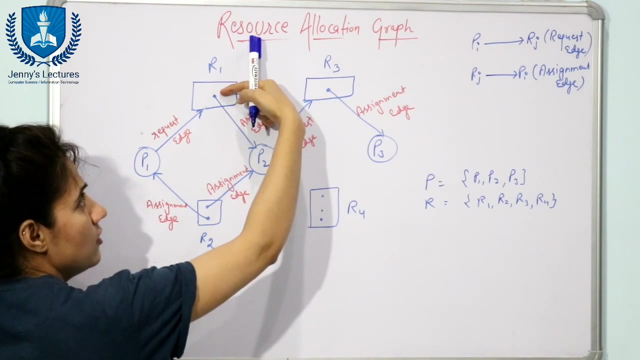 Rectangle, not not. it request edge would not go inside the inside this rectangle. Fine, Request edge would be from process to the box of this rectangle and assignment edge would be from this dot. You can say that instance, instance R1 is having only one instance from the instance of the resource to that process. 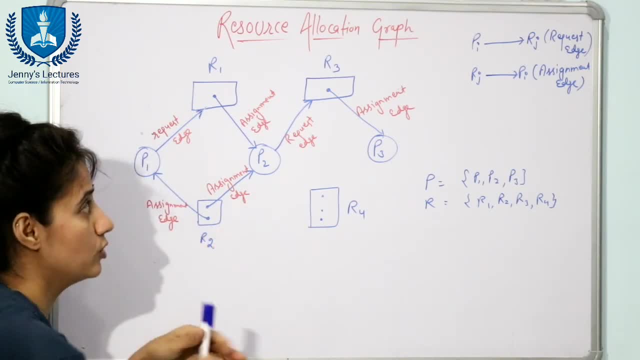 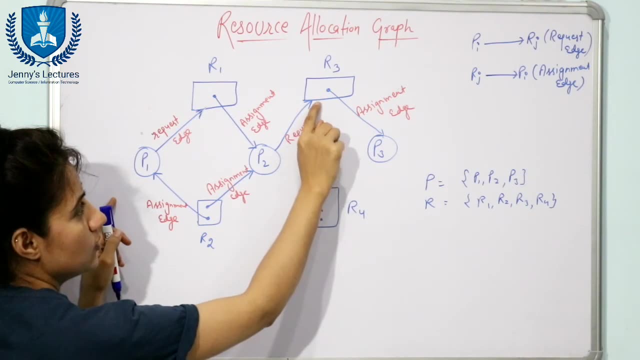 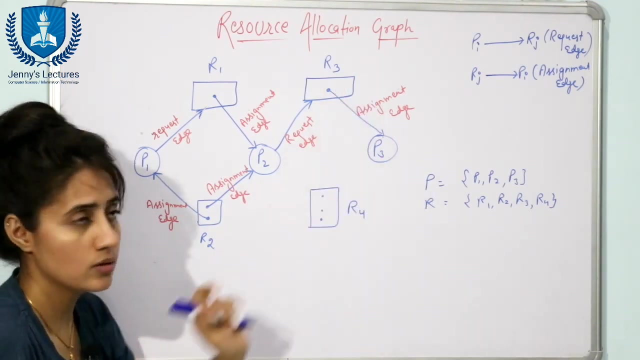 You want to draw this more accurately, then you have to take care of this thing also. See, see. here you can say: all the request is this one and this one are from process to this box, and all the assignment edges are from this door to this process, from this door to this process. 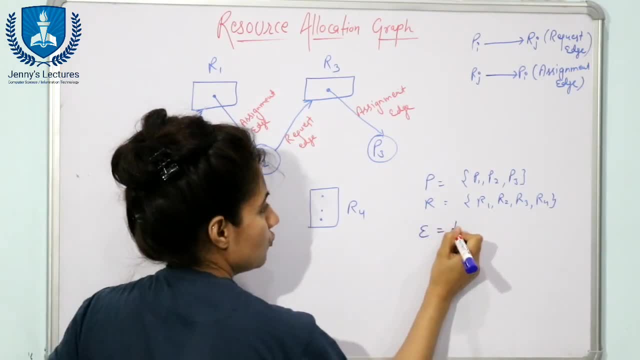 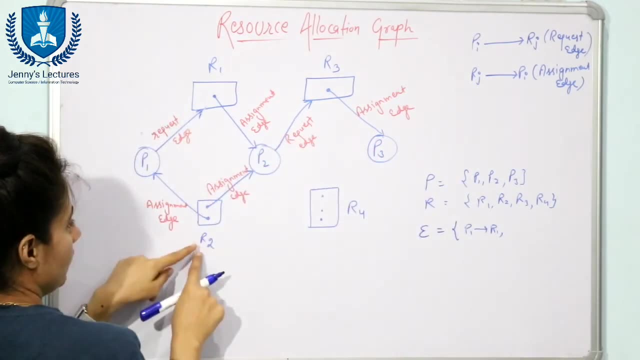 Fine. So here you can say: set of edges would be see P1 to R1, P1 to R1.. Or you can say from R1 to R2.. Or you can say from R1 to R3.. Or you can say from R2 to P1. 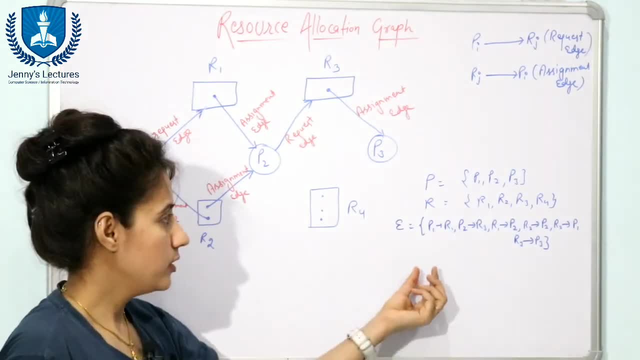 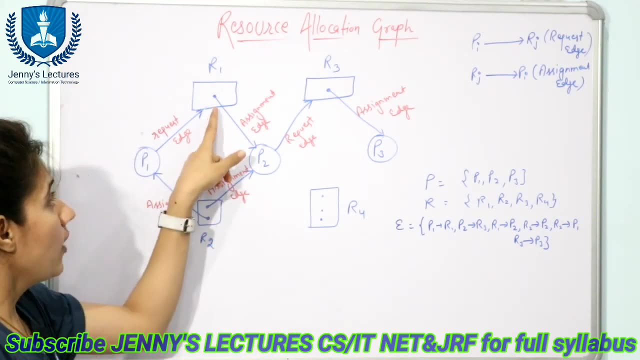 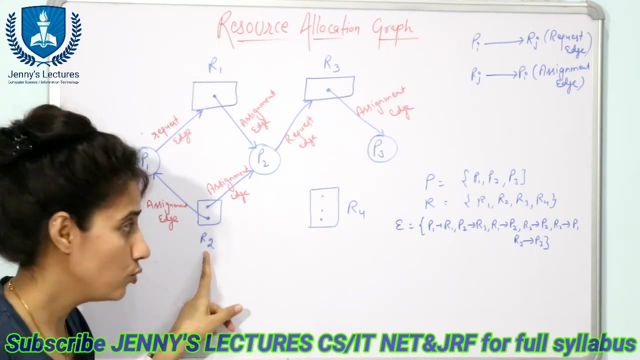 And like this you can write all the edge. So this would be set of edges. Now, if I come to the instances of the resources, then what you can say: one instance of R1, one instance of R3, one instance of- sorry, two instance of the resource type, R2 and 123. 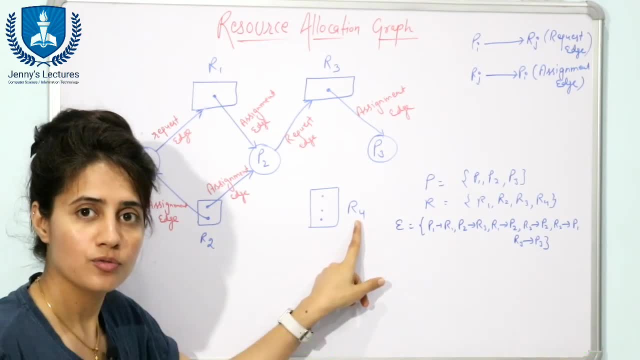 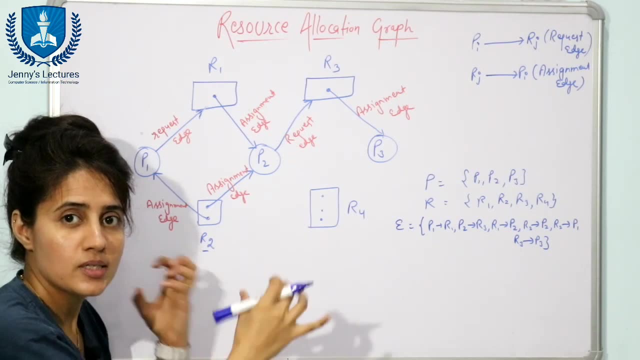 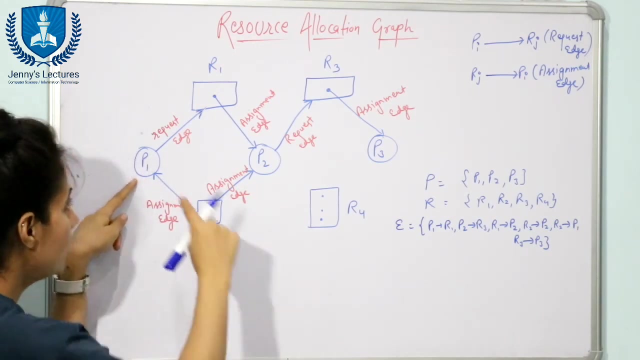 Three instances of resource type R4.. You will find out this diagram in your Galvin book. Next thing is, if you discuss the process states, then here here you can say this process: P1 is, P1 is holding. which resource P1 is holding? 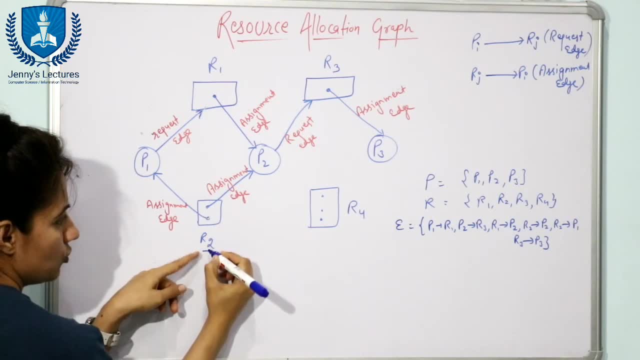 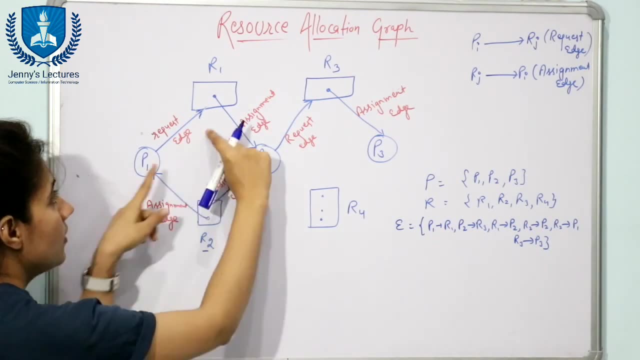 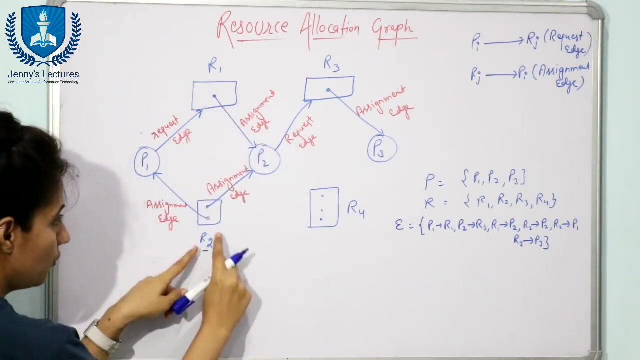 See only one instance. We have two instance of this, R2, but P1 is holding only one instance of resource type R1 and waiting request edge means it is waiting for an instance of resource type R1.. And holding one instance And holding one in the source, resource type R2.. 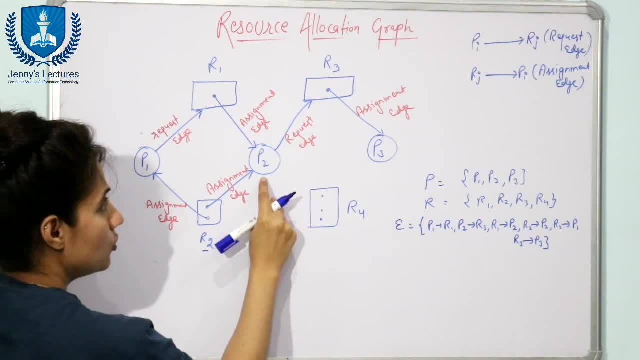 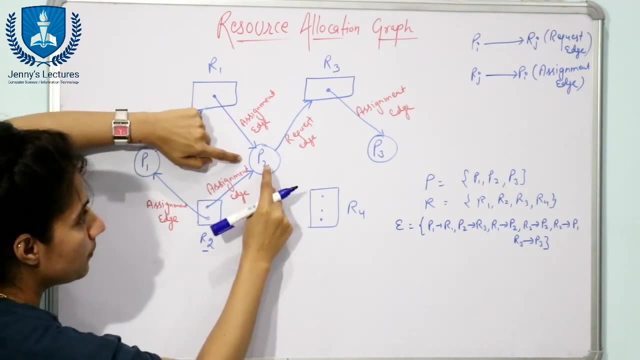 What about P2?? P2 is holding. P2 is holding, See one instance of resource type R1.. One instance of resource type R2.. And P2 is waiting for an instance of resource type R3.. What about P3?? 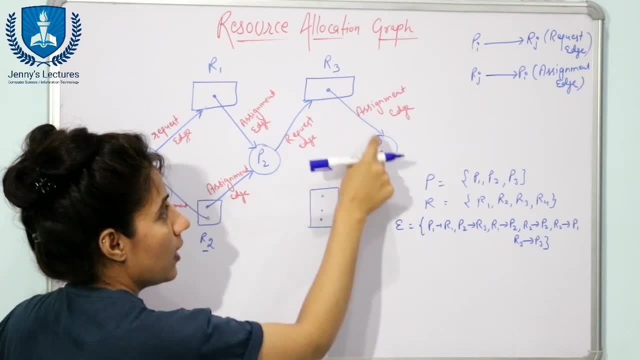 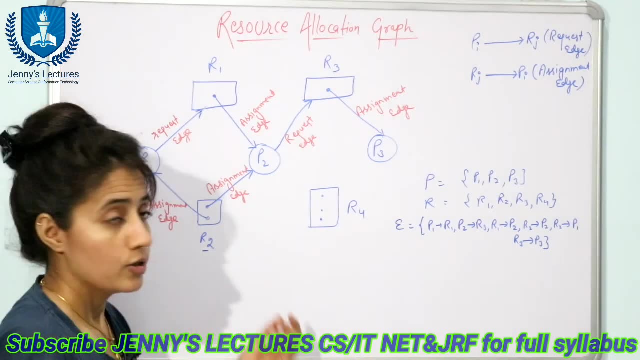 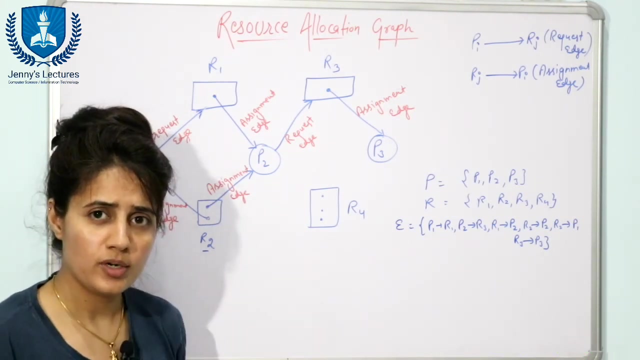 P3 is holding an instance of resource type R3. And obviously P3 is not waiting for any instance. Fine, And this R4 is free. So this is the process states. See, one thing you have to take care of. That is very important thing. 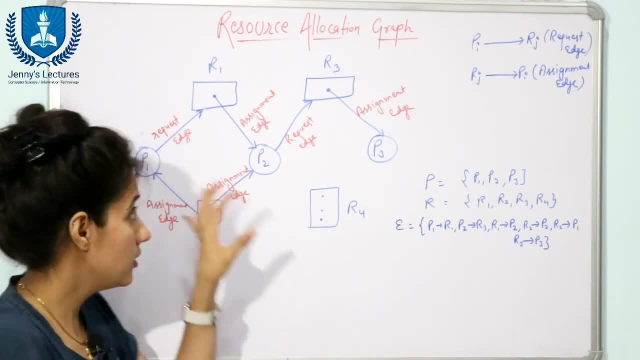 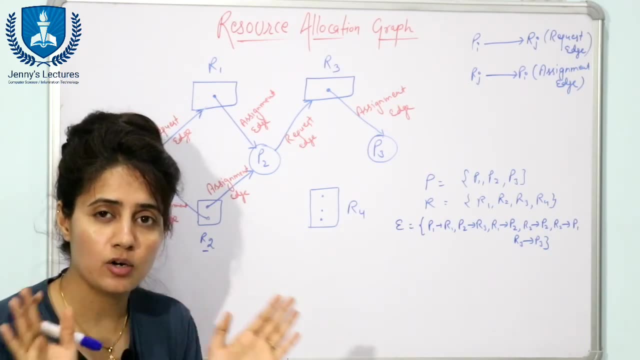 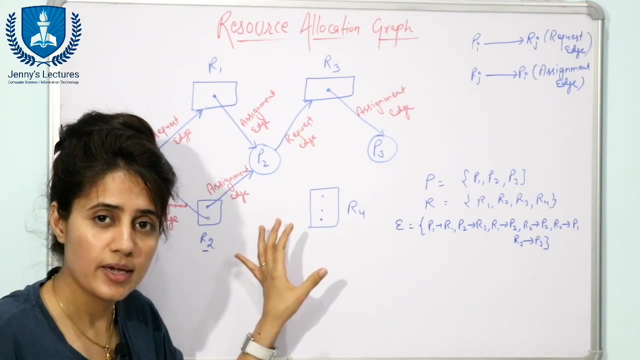 If there is no cycle in this resource allocation graph, Then you can say there would be no deadlock, That no process would be in deadlocked state. Yes, Fine. Second thing is, if, if cycle exists in resource allocation graph, Then deadlock may exist. 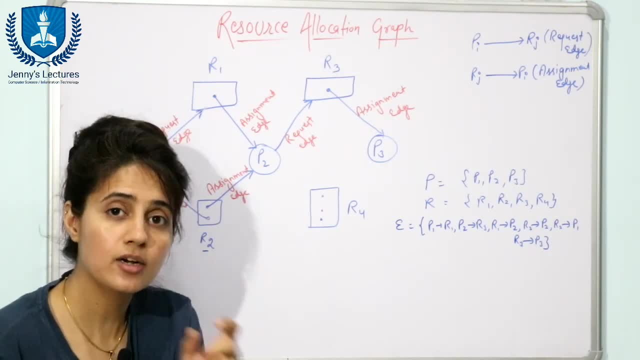 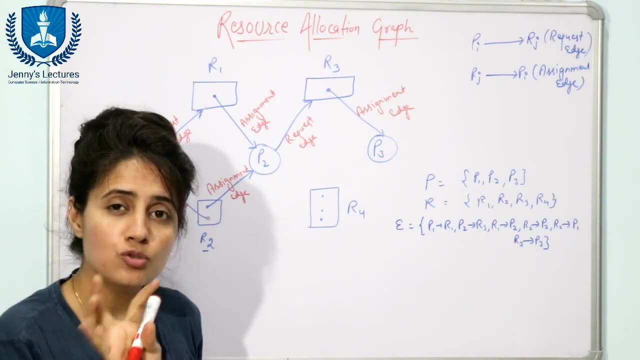 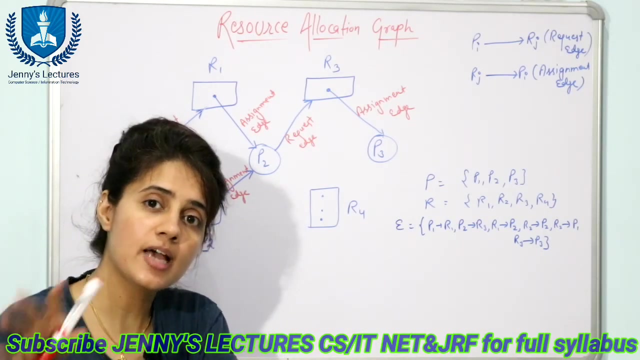 I am not saying deadlock will exist. Deadlock may or may not exist, That depends. We will discuss that thing also. So now we will discuss two resource allocation graph. One graph is having cycle And having deadlock, And second graph, which is having cycle but no deadlock is there. 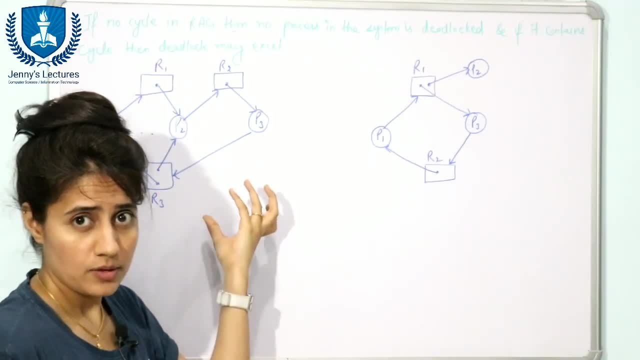 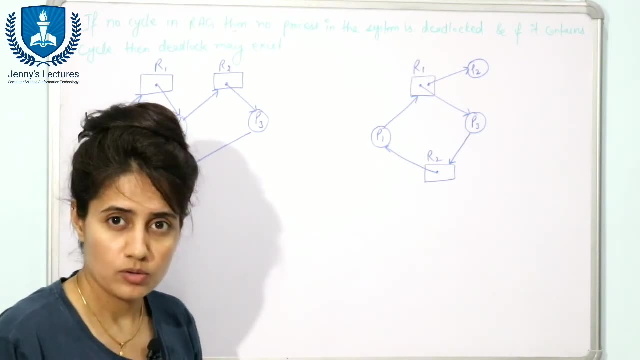 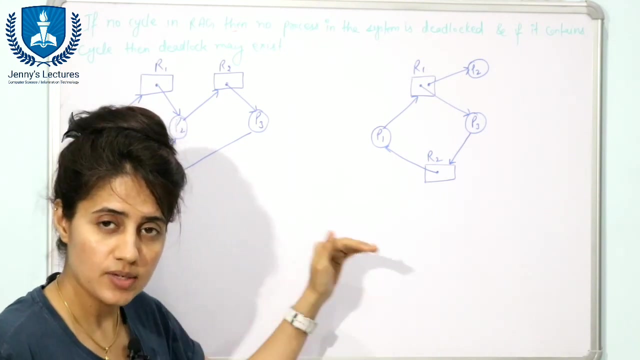 Now, this is the condition. If this, If your resource allocation graph Contains no cycle, Then there would be no deadlock In the system. Fine. And second case is: if cycle it contains a cycle, Then deadlock may exist. See, then deadlock may exist. 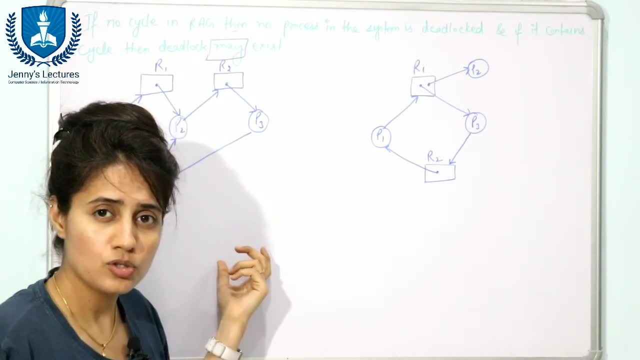 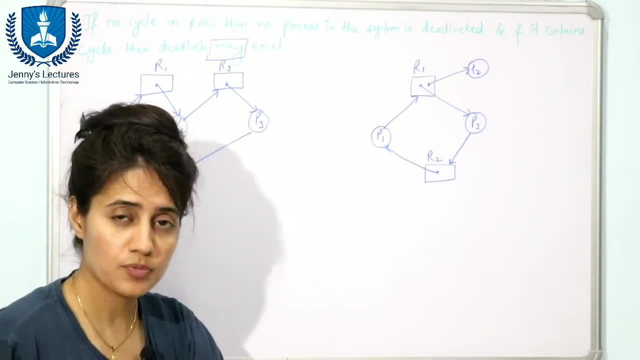 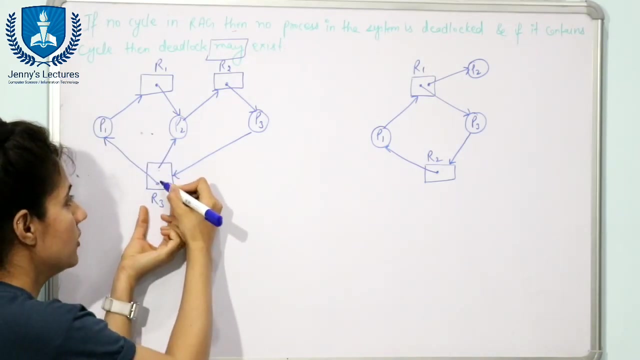 We cannot say that if cycle, if the resource allocation graph contains cycle, Then there would be a deadlock. No, deadlock may or may not exist. Fine, We will discuss this case with the help of these two examples. See this: R3 resource type is having two instances. 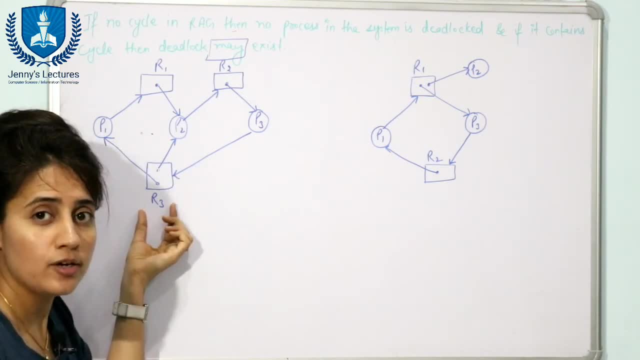 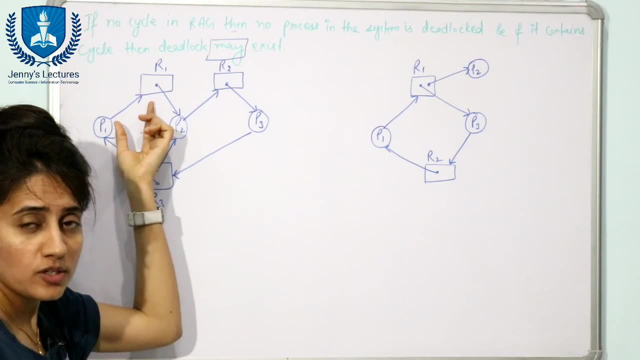 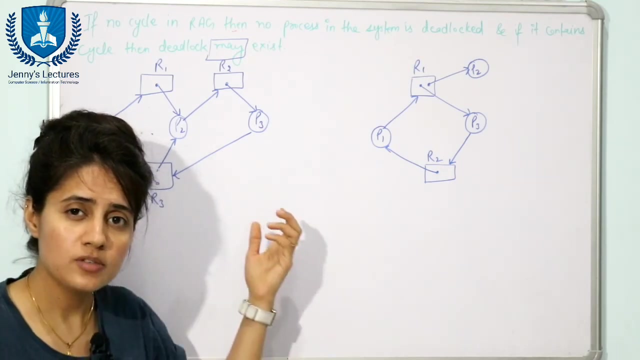 Means at the same time, R3 can be assigned to two processes Because it is having two instances. It is having only one instance, So this resource type can be assigned to one process at a time. Okay, Now how you will check from this resource allocation graph. 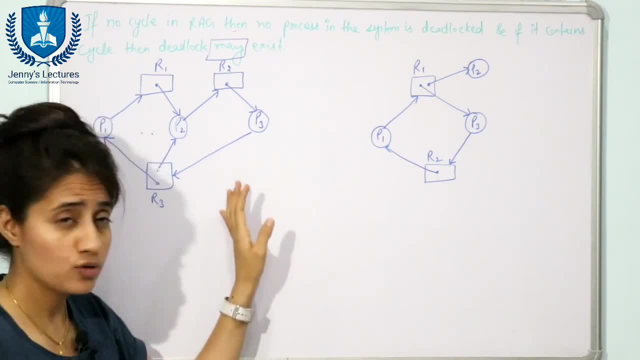 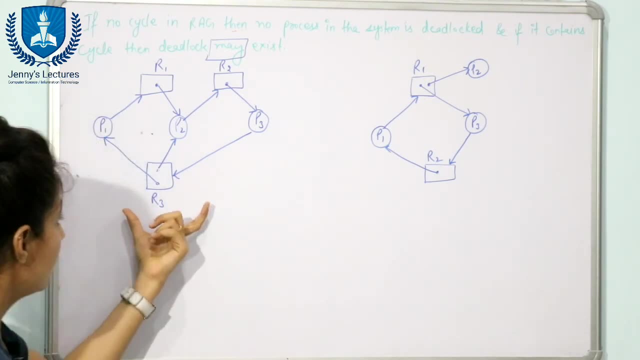 That the system is having deadlock or not. If small resource allocation graph is there, Then you can check it just by looking at this graph. See, when you are looking at this graph, Then it if first of all check if this graph contains a cycle or not. 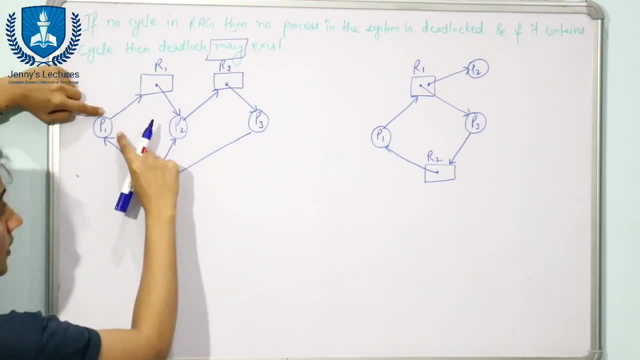 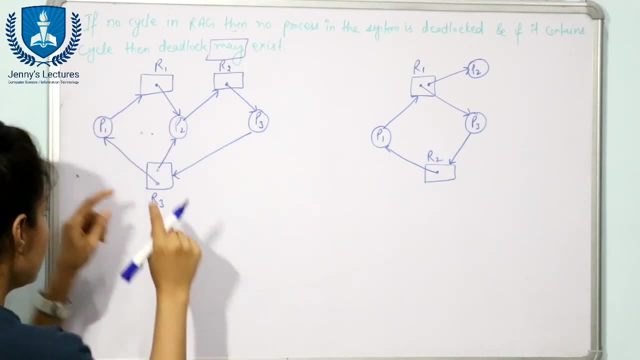 Yes, this contains a cycle. It is having two cycles. One is this: one Cycle means so you can say closed path, You will start from one point and you will reach out to that point. only See, we will start from P1.. This one, P1 to R1.. 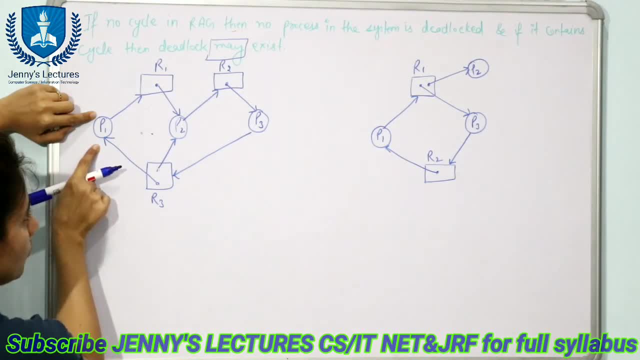 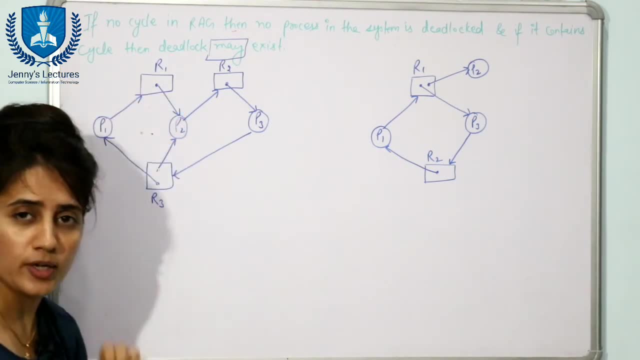 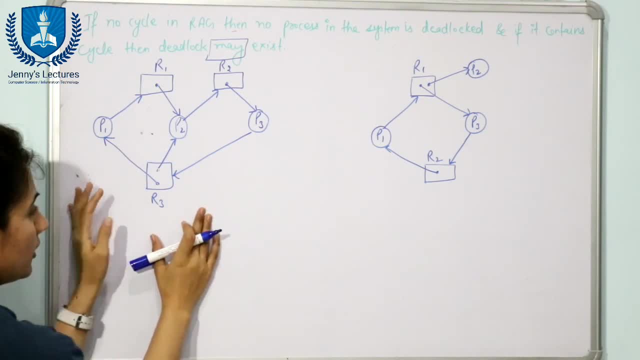 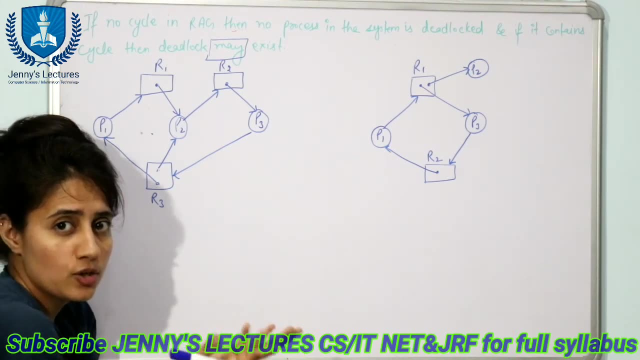 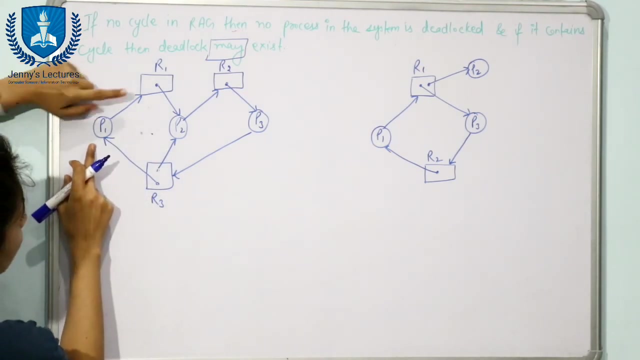 May or may not. Now how to check. If first of all you check, is there any process? who is in the state of progress Or who can execute? Who can complete its execution? Check for P1.. P1 is waiting for R1.. 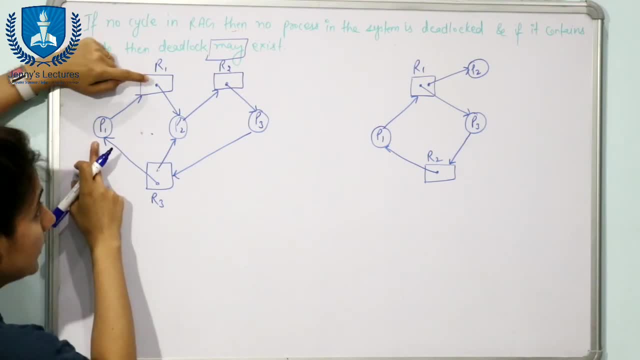 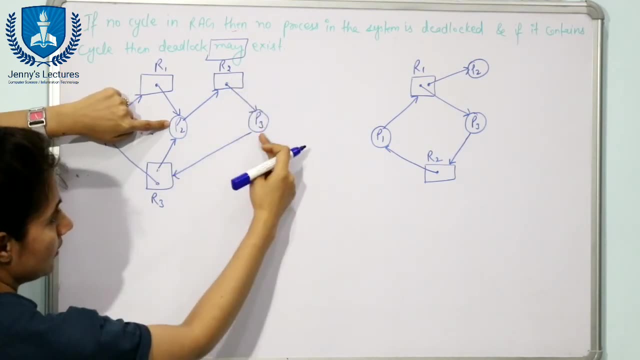 So P1 cannot execute Till it gets R1.. P2.. P2 is waiting for R2.. But R2 is held by this P3.. So P2 also cannot execute P3.. P3 is waiting for this R3. 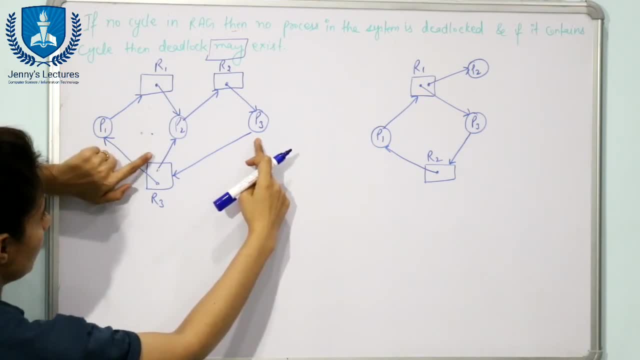 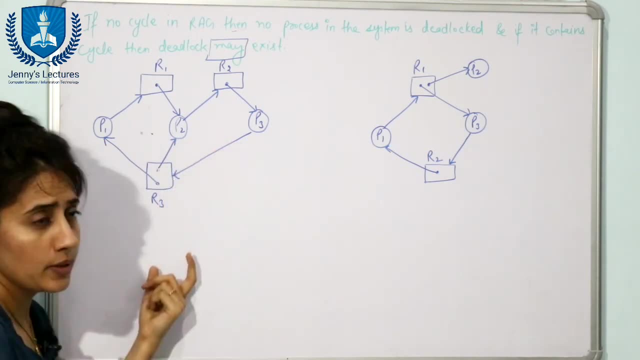 But this R3 is held, One instance is held by P1.. One instance is held by P2. And these both are also in waiting state. So neither P1 nor P2 nor P3 can execute. So here is no progress. 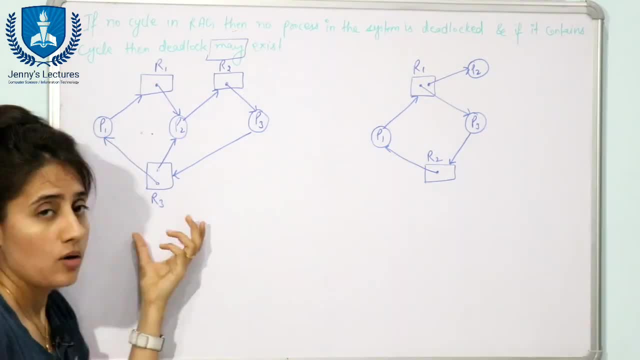 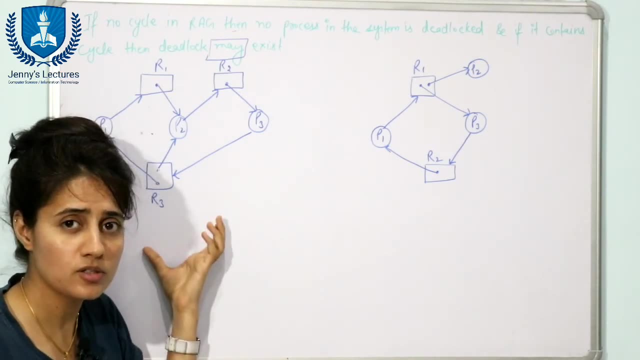 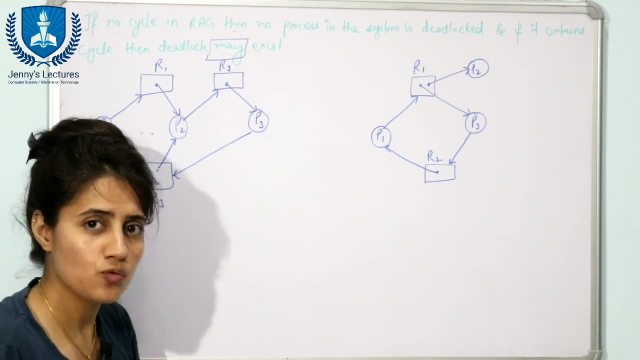 So you can say this is a deadlocked state. Or second way is: If complicated resource allocation graph is given, Then just by simply looking in this graph, On this resource allocation graph, You cannot say that it is having deadlock or not. So second method is what? 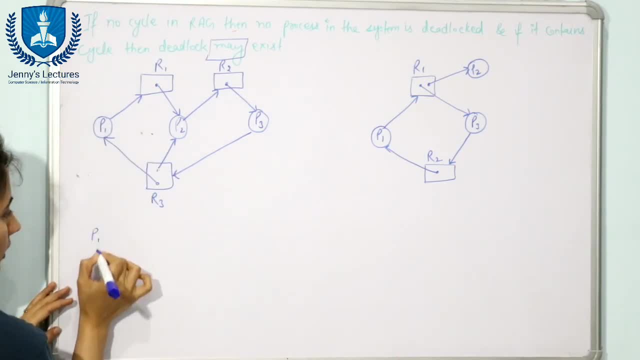 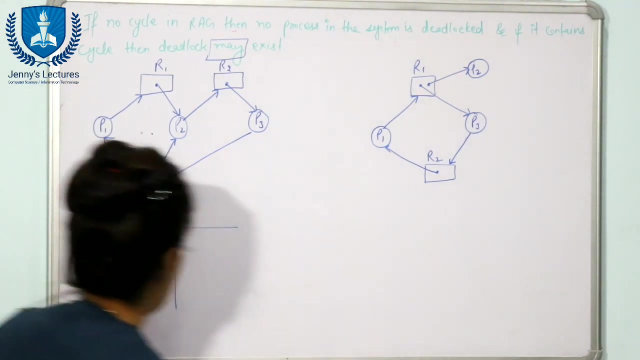 Simply write down how many processes you have: P1., P2. And P3.. Right Now, resources are R1., R2. And R3.. Now it Here. Here we will write, Here we will write allocation. 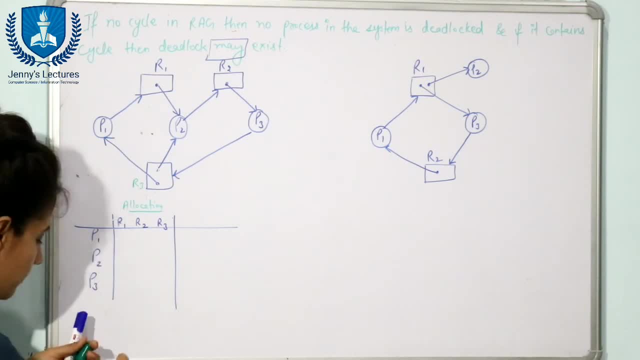 This is you know. you can see allocation matrix. Fine How many resources or which resource is allocated to which process. Check out from this resource allocation graph P1.. See P1 is holding which resource, One instance of this resource type R3.. 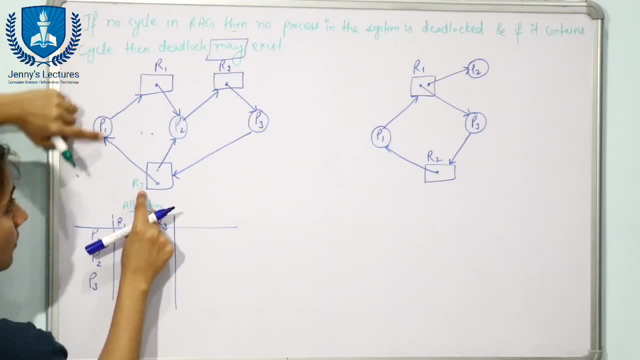 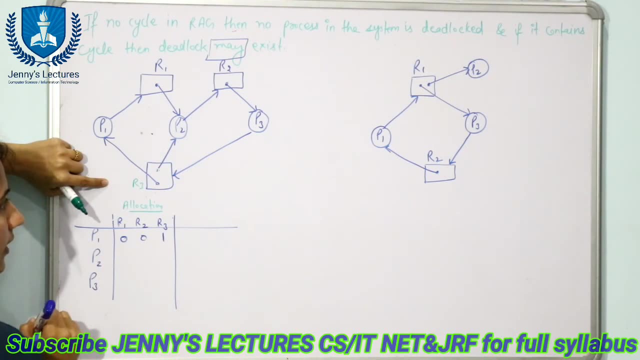 Only this R3.. Because P1 is waiting for R1.. This is only the assignment edge, So R3, you will write 1.. R2 and R1: you will write 0.. Because P1 is not holding Any instance of R1 and any instance of R2.. 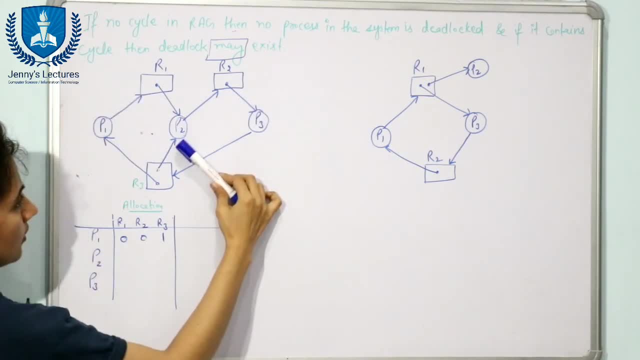 Now check out what about P2.. P2 is holding. P2 is holding Only one instance of R3.. One instance of R3.. P2 is holding Plus. P2 is also holding one instance of R1.. From this RAG: 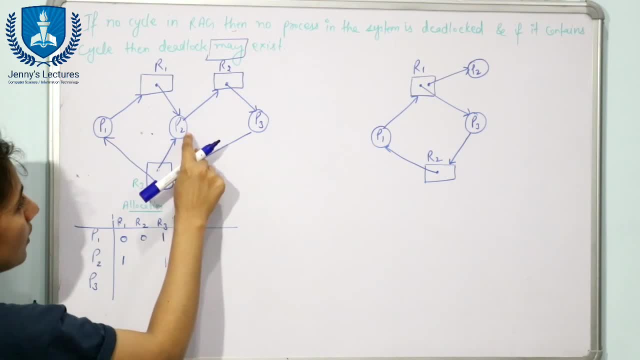 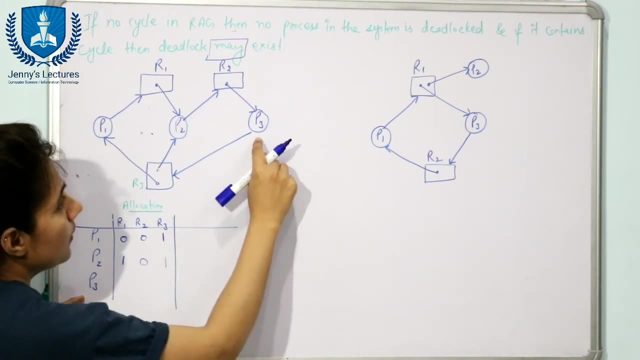 From this resource allocation graph, You can easily analyze this thing. P2 is holding R2.. No, P2 is not holding R2.. P2 is requesting R2.. Now what about P3.. P3 is holding. P3 is holding only one instance of R2.. 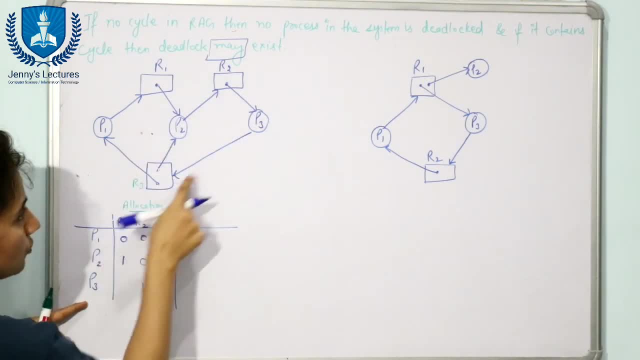 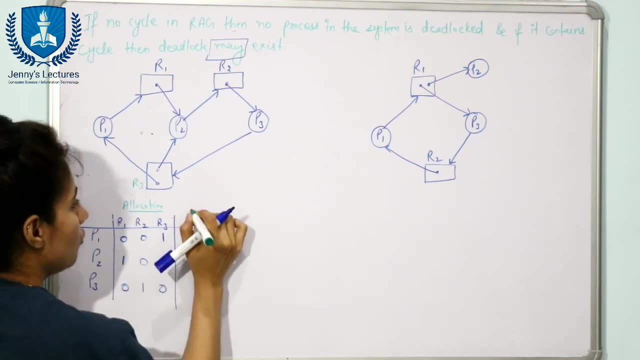 R2.. R1. No, R3. No, P3 is waiting for R3.. So 0 and 0.. So this is the allocation matrix. Now we will write down the request matrix. Or you can say: need matrix. 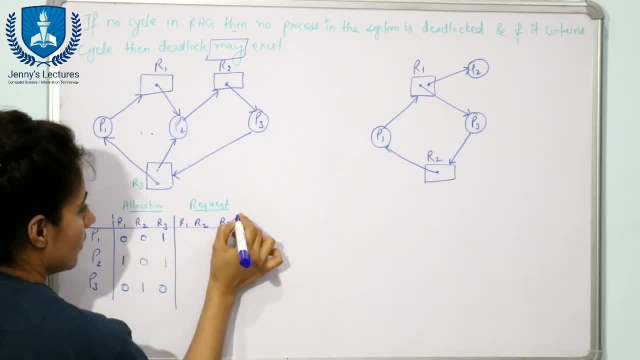 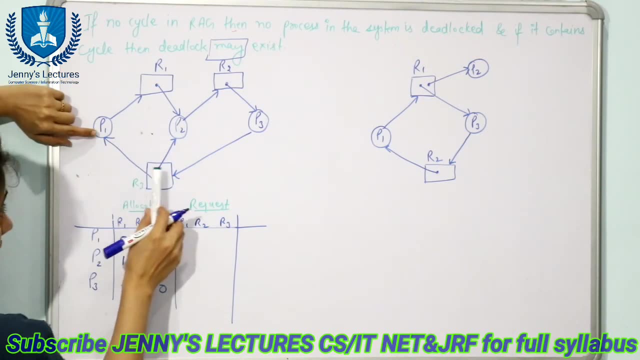 For this: R1.. R2 and R3.. What is the request matrix of P1.. See, From this graph you can easily check P1 is requesting R1.. One instance of R2.. One instance of R1.. Right. 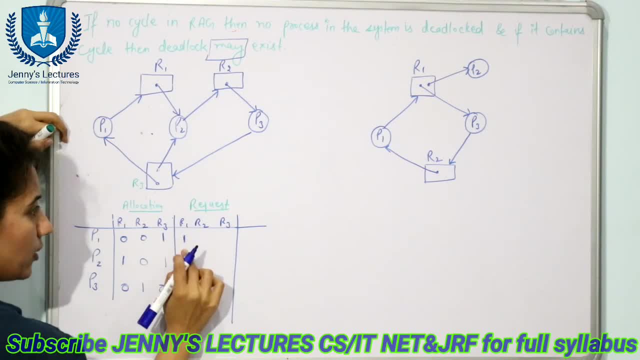 P1 is requesting R1.. Requesting hai, It means you will write: 1. P2 is requesting R2.. No, Is P2 requesting R3.? No, Now what about P2.. P2 is requesting What? P2 is requesting R2.. 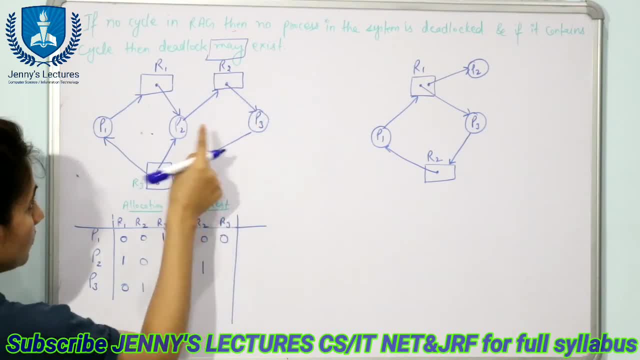 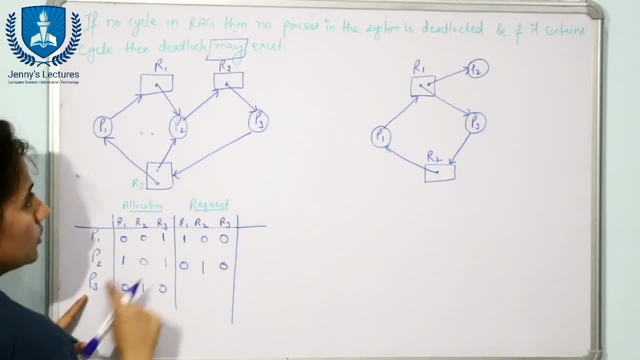 P2 is requesting: See, this is requested R2.. Is P2 requesting R1.. No. P2 requesting R3.. No 0 and 0.. What about P3.. See, P3 is requesting only R3.. R3. 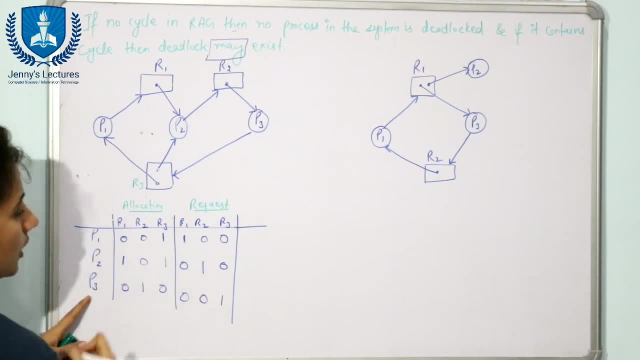 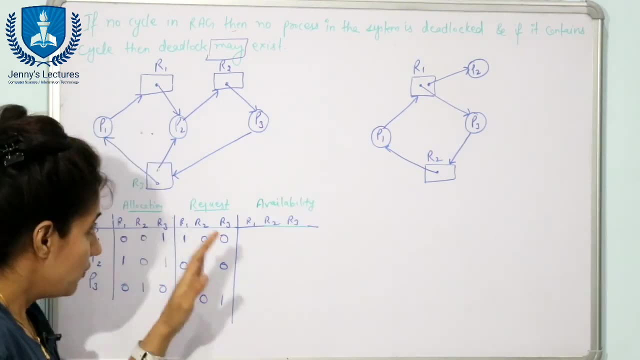 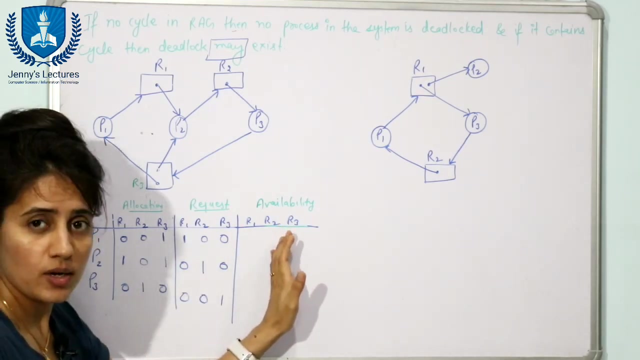 P2 is not requesting R2.. Sorry, P3 is not requesting R1.. Fine, Now What is available matrix. we have Availability. After the allocation of This, This: These Resource type: How many resources are still available with us? 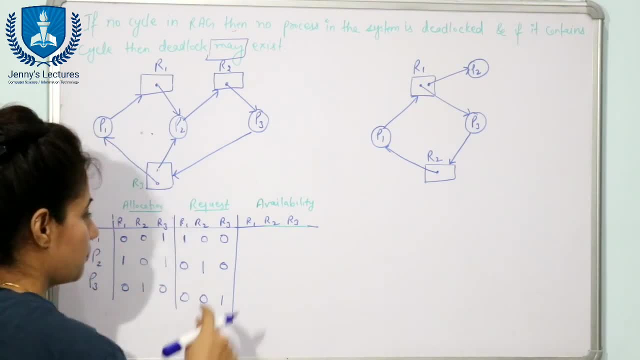 How many instances of these resource types are available with us. See, R1 is having only one instance and this is allocated to P2.. So we don't have any instance of R1.. R2 is having only one instance and this is allocated to P3. 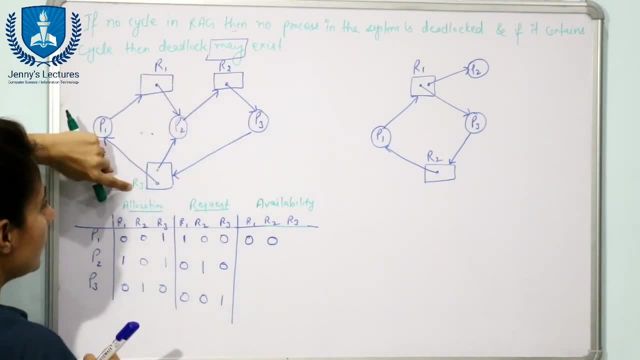 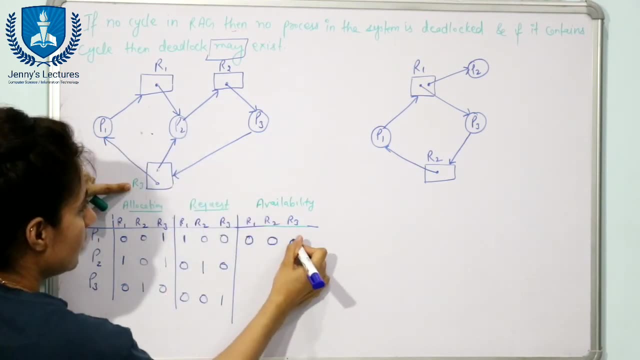 So we don't have any instance of R2 available. R3. See, R3 is having two instances and both are allocated to 1 to P1 and 1 to P2.. We don't have any R3. So availability is 0, 0 and 0. 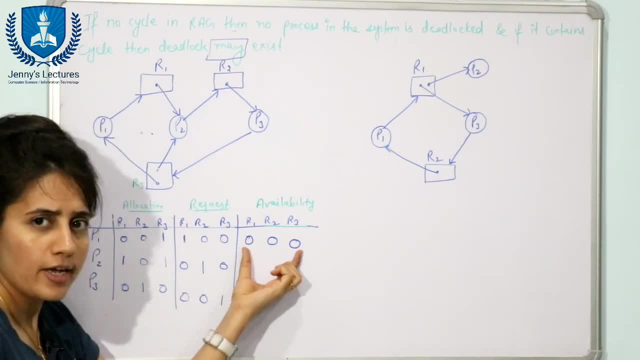 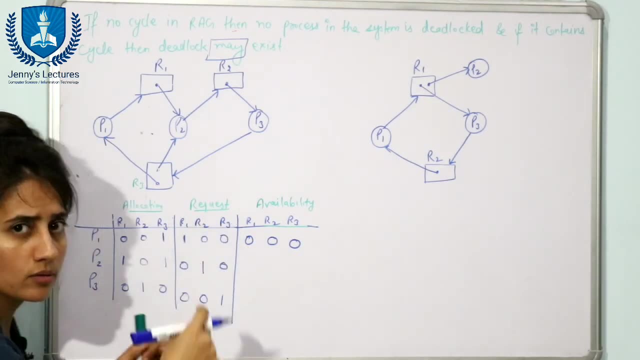 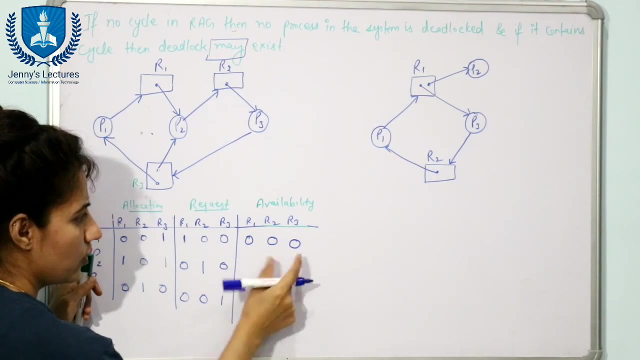 Now, with this availability, Can you fulfill the requirement of, or you can say need of, any process? Check out the request or need. matrix of P1.. 1 0- 0.. P1 need one instance of R1 but we cannot fulfill with this availability. 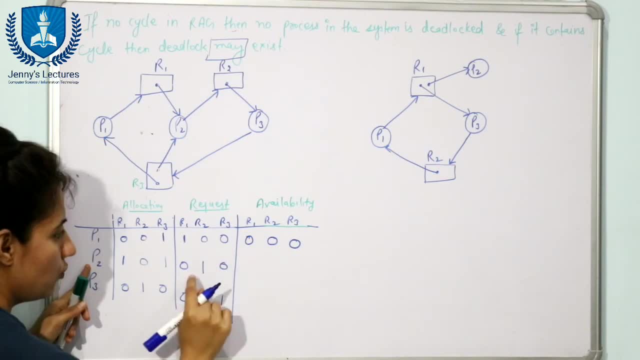 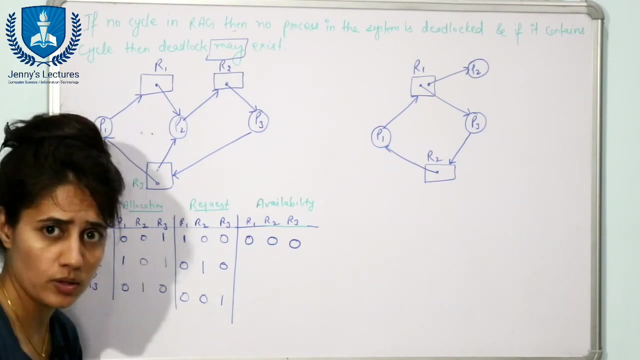 P2 is requesting 0 1 1, but we cannot fulfill this request with this availability. P3 is requesting 0 0 1, but we cannot fulfill this request with this availability. So We cannot fulfill request of P1, P2 and P3.. 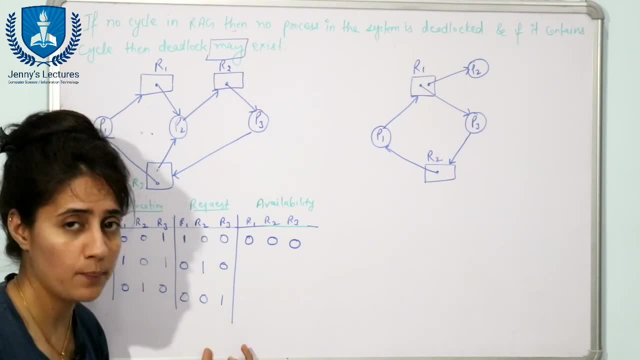 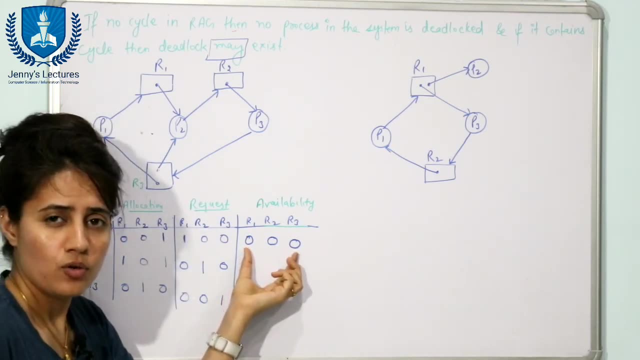 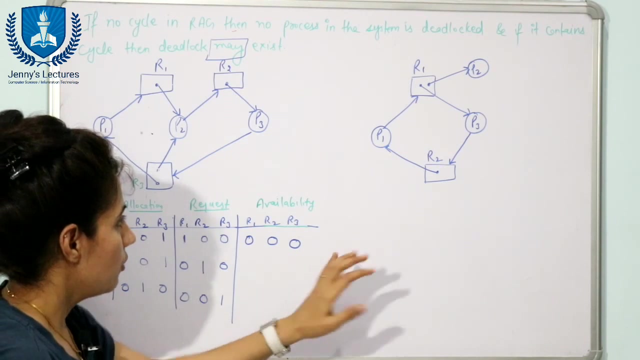 It means no process can execute, can complete its execution. It means here we have no progress Because we have 0 availability of all the resources. It means this: this system is in deadlocked state. Now check out with this one See this contains a cycle or not. 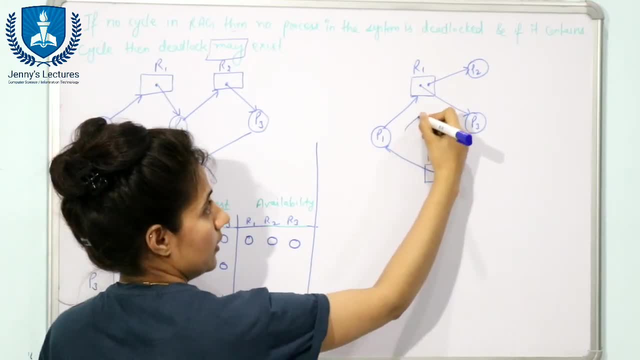 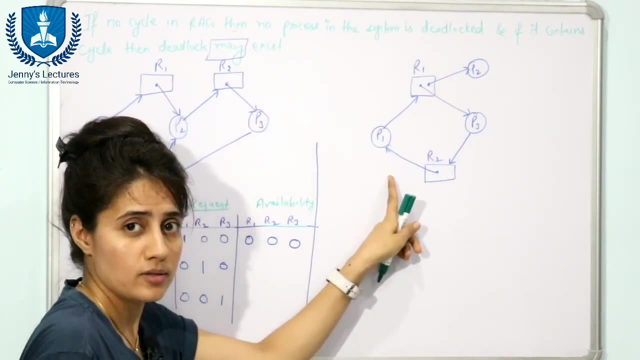 Yes, this graph contains a cycle. This one, Yes, this one, This one, This one And finally to this one. So this is a cycle, But it doesn't mean that it also contains it also. This system is also in a deadlocked state. 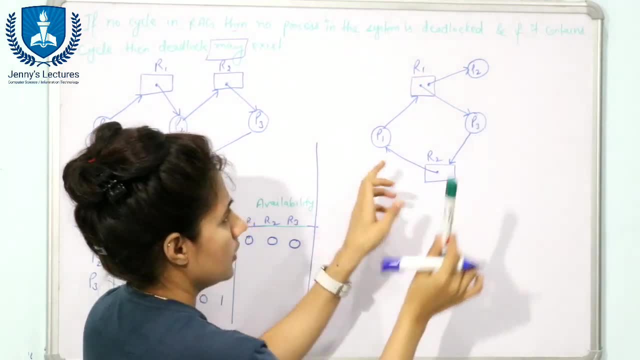 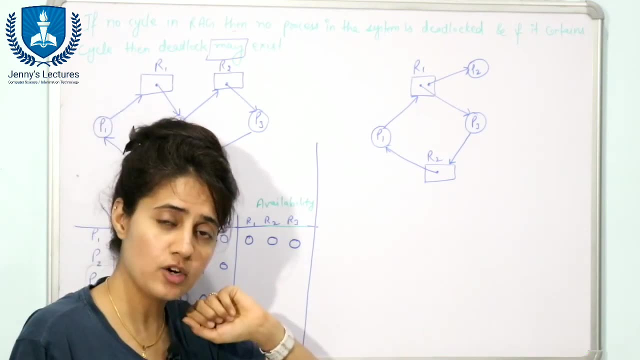 You have to check it out. We have P1, P2 and P3.. Which process is in the state that it can execute? it can complete its execution. Check out First of all. check out which process is not waiting for any resource. P1 is waiting. 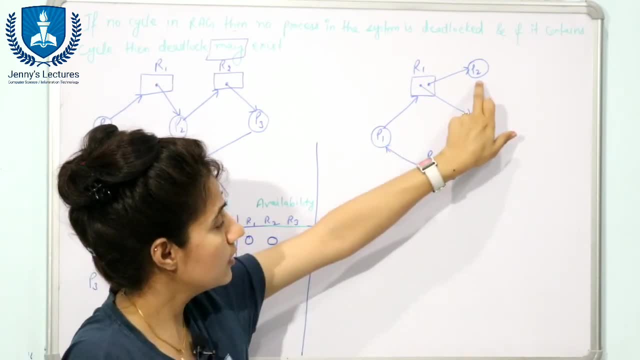 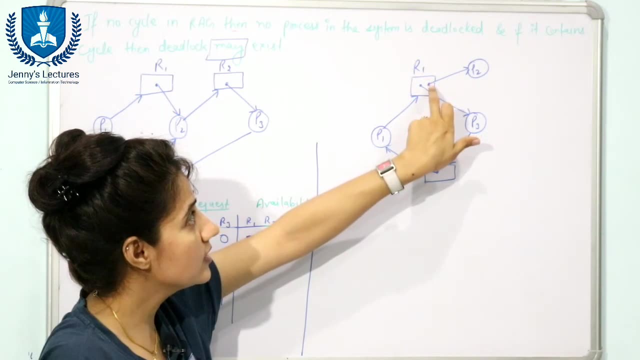 Yes, P3 is waiting. Yes, P2. is P2 waiting for some resource? No, P2 is not waiting. P2 is holding one instance of R1.. Here we have two instance of R1, one instance of R2.. P2 is not waiting for anything. 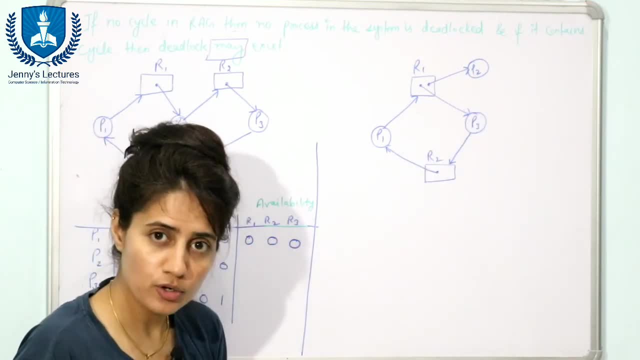 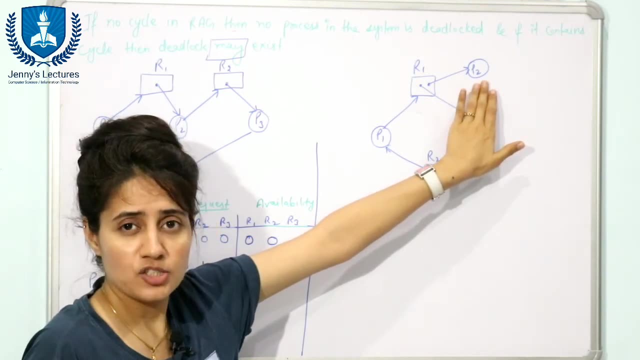 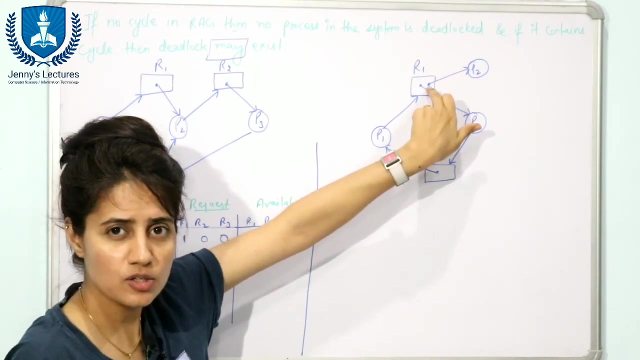 It means P2 can complete its execution at some point of time. If P2 is not waiting, Fine, And after P2 finish finishes its execution, Then This P2 will release This instance Of this resource R1.. It means: 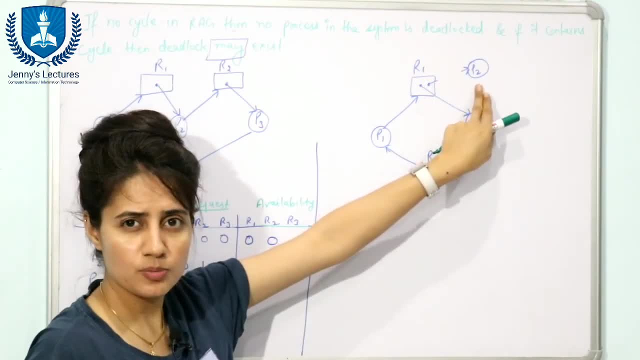 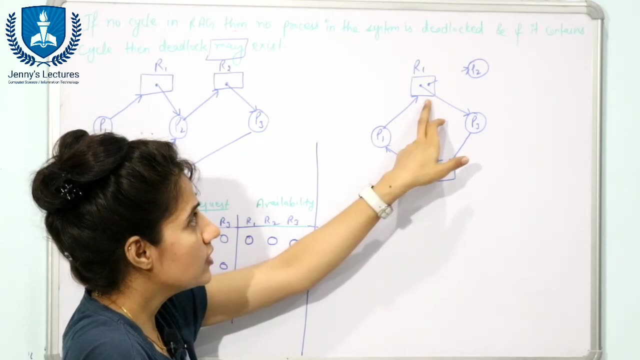 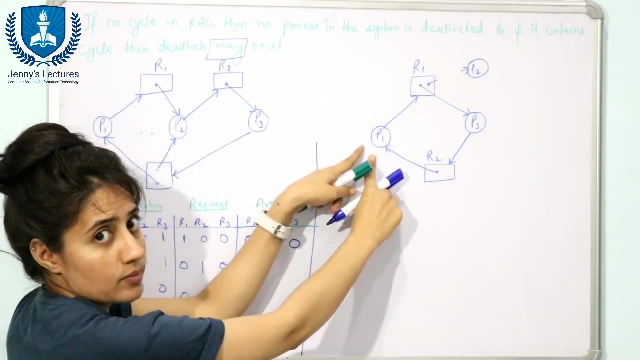 You can delete this edge after the completion Of this P2.. Now this resource is available. Now one instance of R1 is available. Now see P1 is requesting Instance of R1.. Now we can allocate this one instance to P1.. 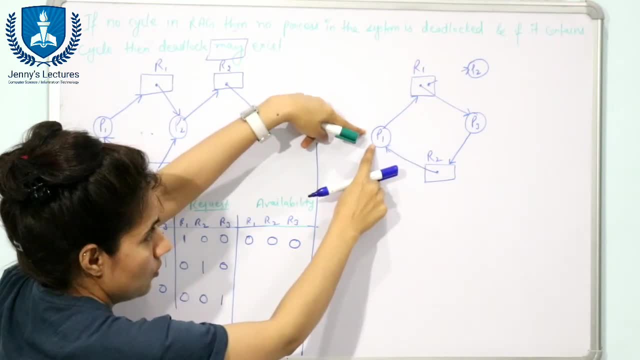 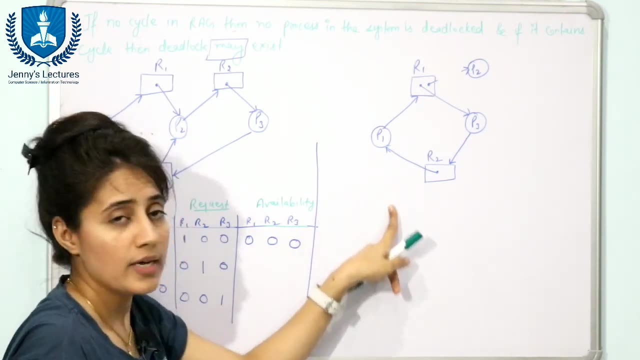 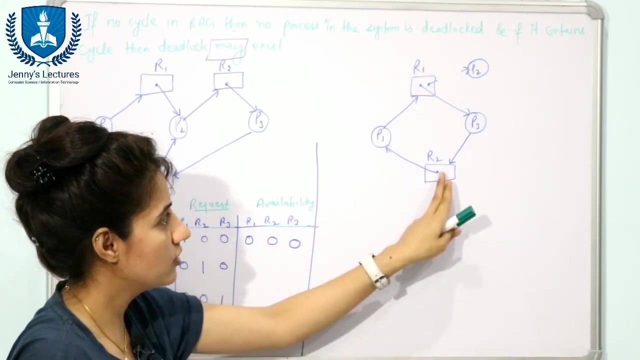 Now, after: after this allocation of this R1.. P1 is now Not waiting for anything, Fine, So P1 can complete its execution Now. after completing this execution, P1 can release this instance. P1 can release this R2 also. 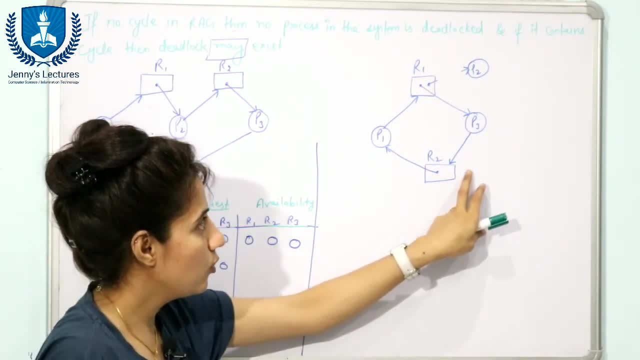 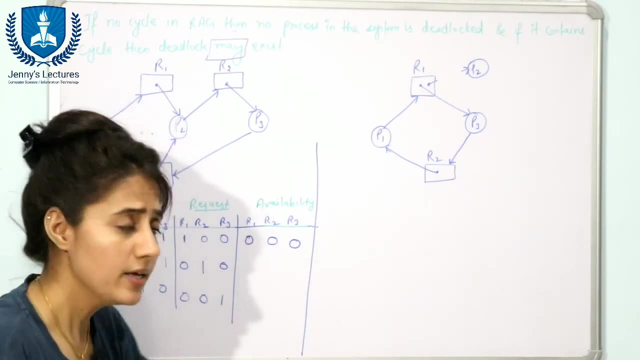 Now, if R2 is free, Then this R2 can be allocated to P3.. Now, P3 now can complete its execution And system is not in deadlock state, And if you check out This with the help of this method, Then you can easily check it out. 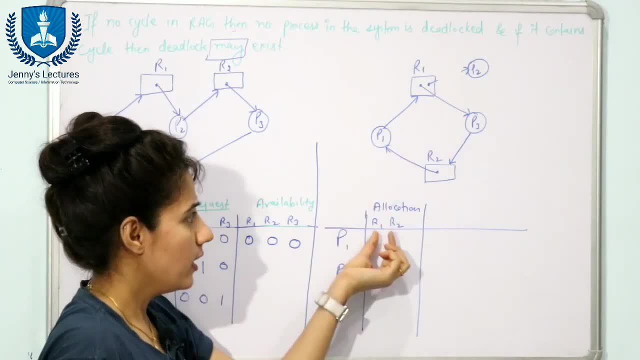 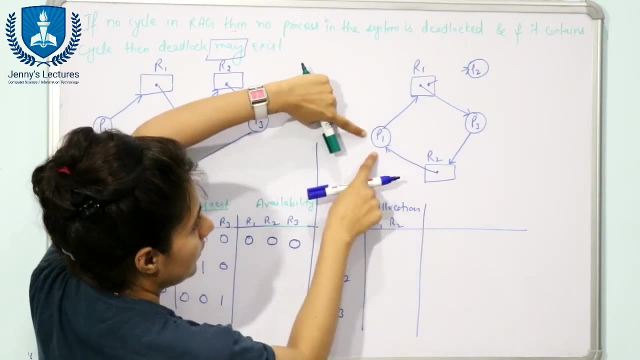 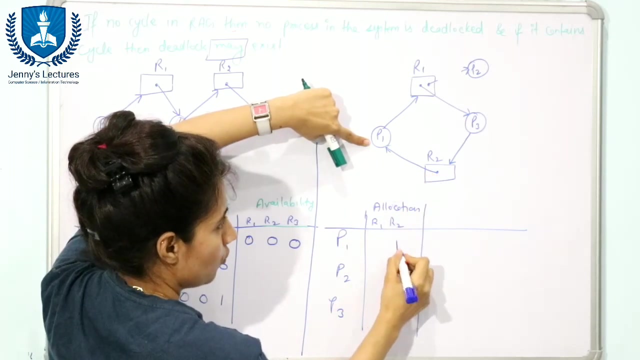 Here we have only two resource type: R1 and R2.. Now Now fill this allocation matrix P1.. P1 is holding which resource. Which resource is allocated to P1.. See this: R2.. Means 1.. But P1 is requesting for R1.. 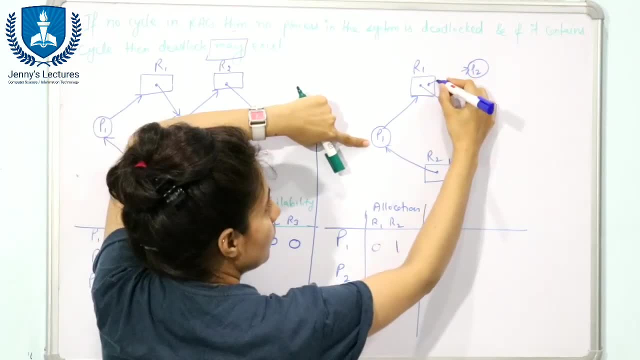 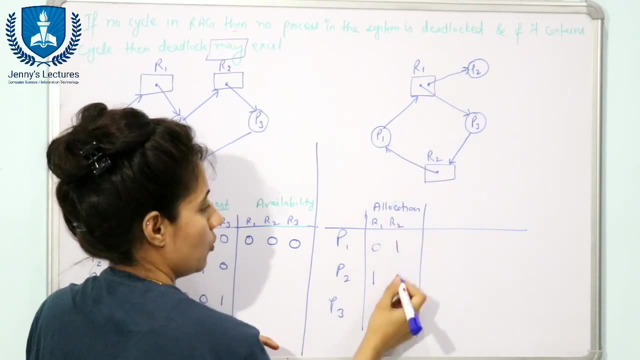 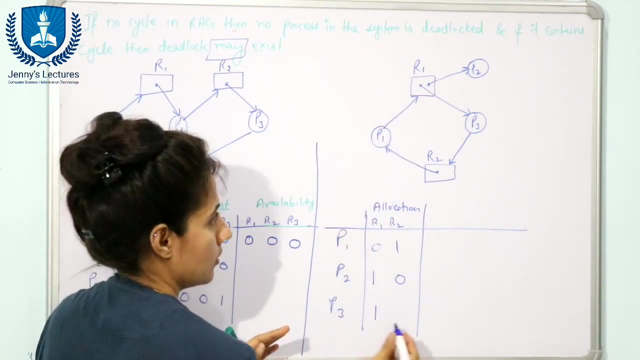 So here we will write 0.. What about P2.. P2 is holding which resource? R1. R1 only. What about P3.. P3 is holding which resource? One instance of R1.. And here we have About R2.. 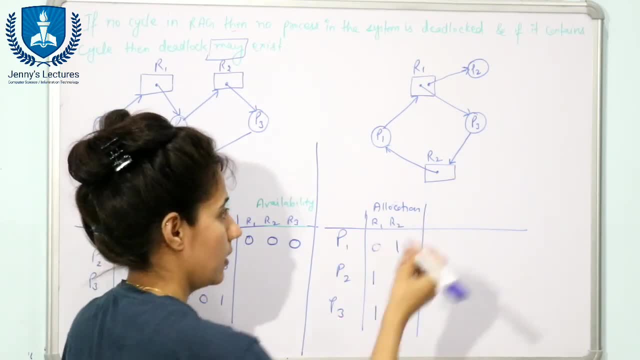 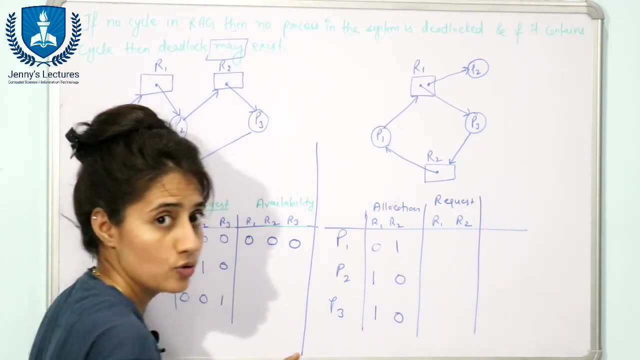 P3 is not holding R2.. That is why we have written 0 here. Now what about request matrix? Or you can say need matrix R1 and R2.. Check: P1 is requesting. P1 is requesting Which resource? 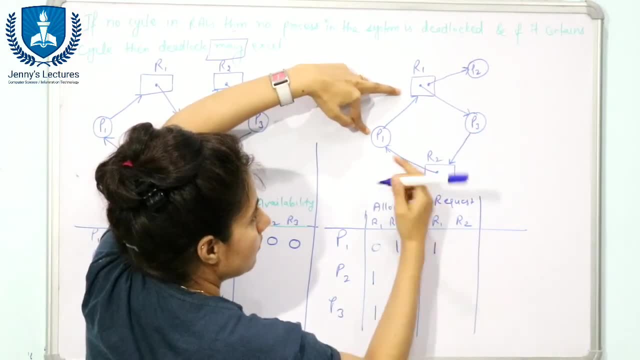 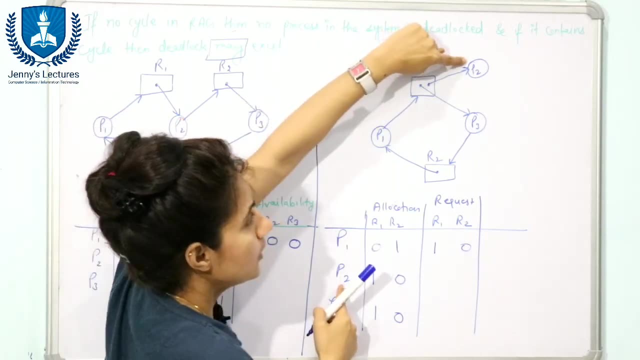 Only this one. R1 for R1.. P1 is P1 requesting R2.. No 0.. Because this is assignment edge. What about P2.. P2 is requesting For Nothing, Neither for R1.. 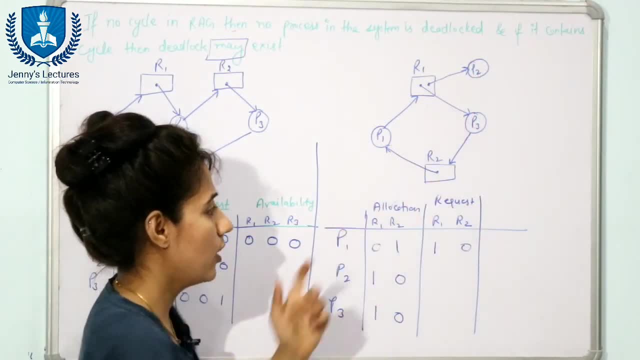 Neither for R2.. So you will write 0 and 0 here, Because there is no request edge. Only one assignment edge is there. What about P3.. P3 is requesting for R2.. So he will write 1.. 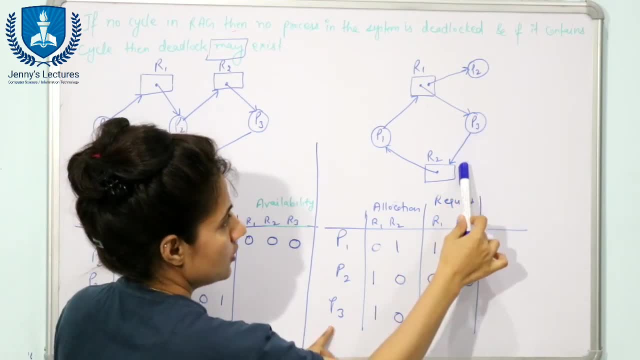 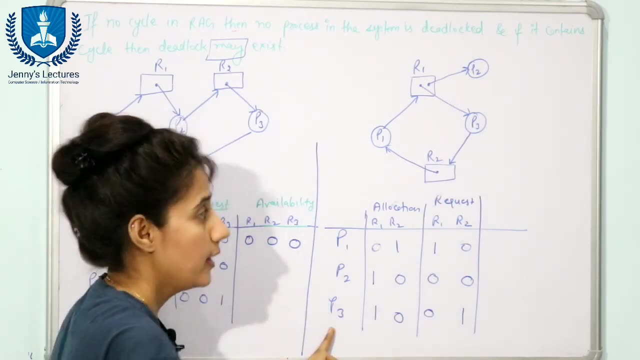 And 0 here, Because there is no request edge. Only one assignment edge is there. What about P3.. P2.. So he will write 1.. Is P3 requesting for R1.? No, Now, What is the availability? 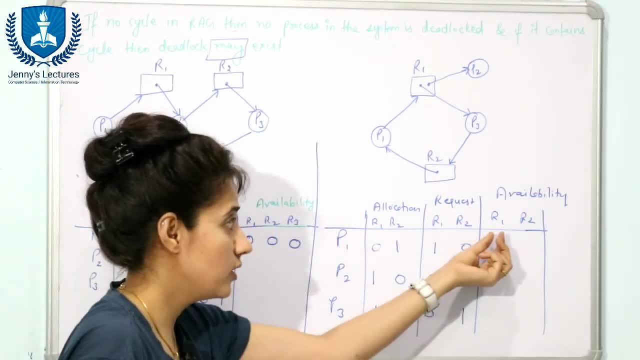 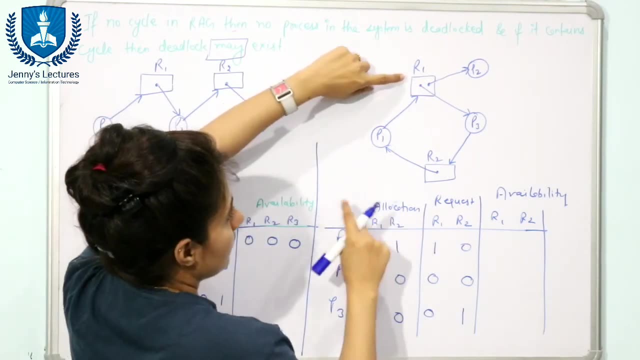 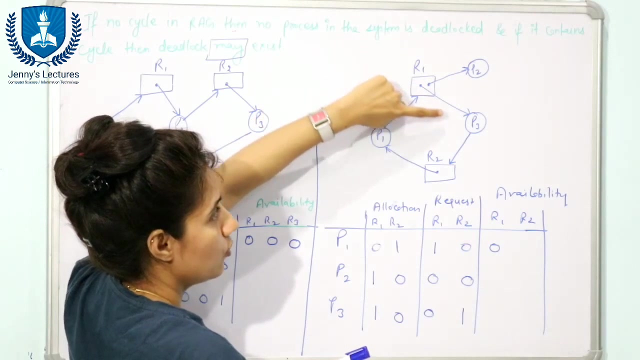 You have to check How many. How many instances of these resource type are available with us After this allocation? Fine, Now See: R1 is having two instances, But no Nothing is available. 0.. 1 is allocated to P3.. 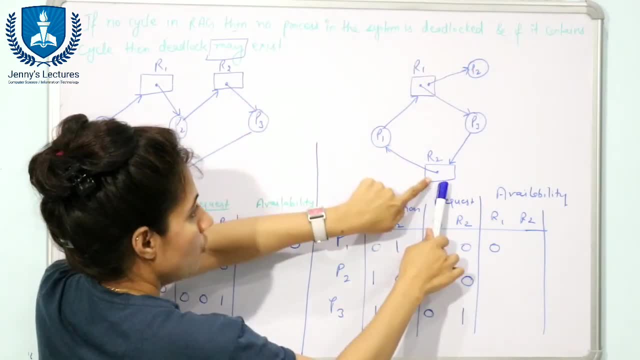 1 is allocated to P2.. What about R2.. R2 is having one instance, And this one is allocated to P1. So we don't have any R2.. So here also, availability is 0 and 0.. Now check out. 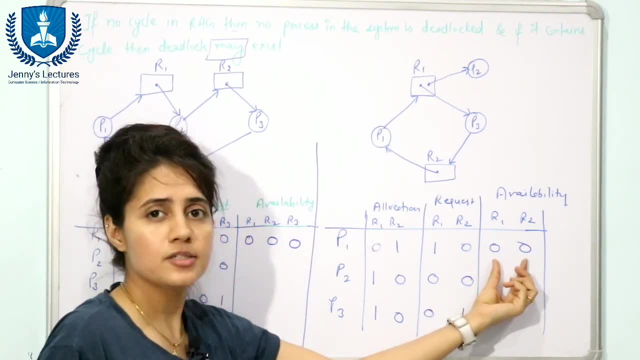 With this availability, Can you fulfill the requirement of any process? Check out the request of these: P1. Request is 1 and 0. But we don't have R1. So we cannot fulfill this request, P2.. P2 is having request of. 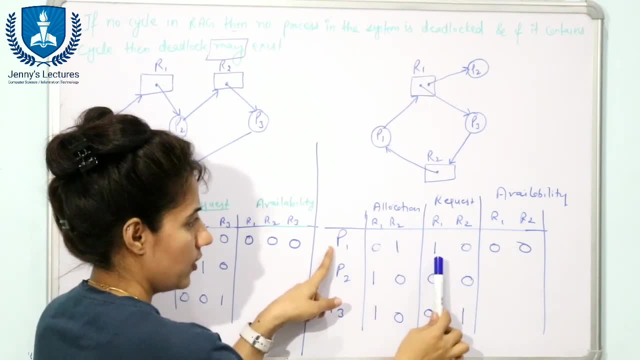 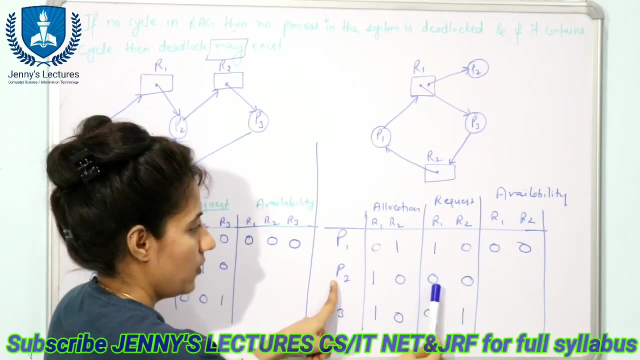 1. And 0. But we don't have R1.. So we cannot fulfill this request. P2.. P2 is having request of 1. And 0.. Yes, That availability is also 0 and. 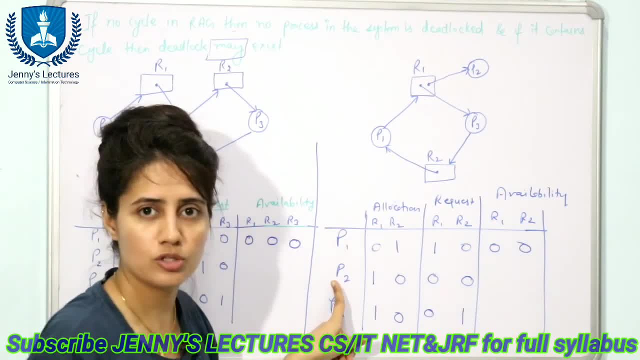 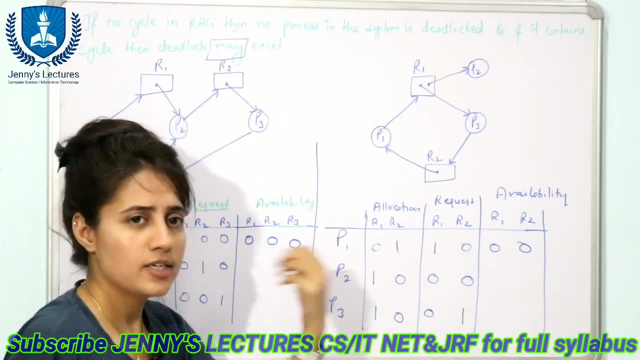 0. Means You can fulfill this request, P2. Request. If you can fulfill the P2. Request, It means at some point of time, P2. Will complete, Complete its execution, Fine, And It will release. 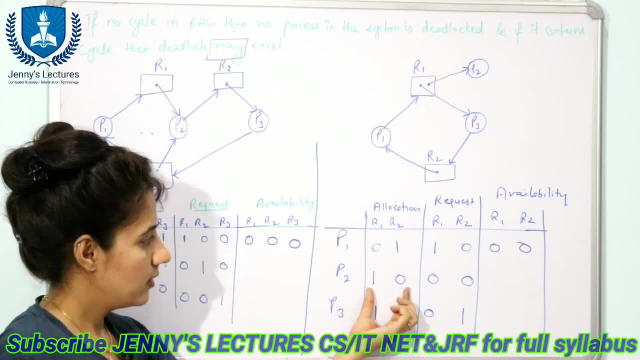 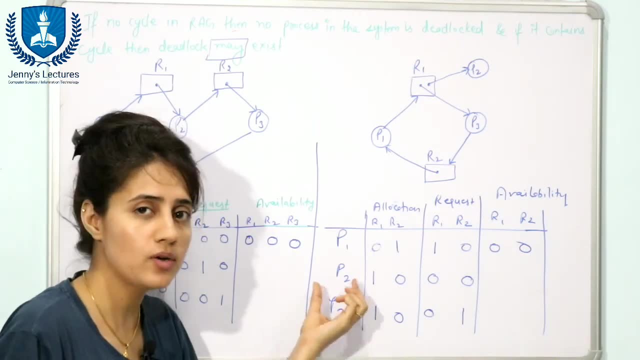 These resources: 1. And 0.. The number of resources which are allocated to P2.. After completion, It will release those resources: 1. And 0. And 0. And 0. So it will release. 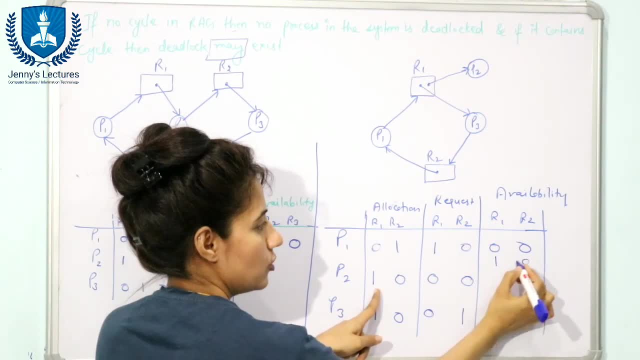 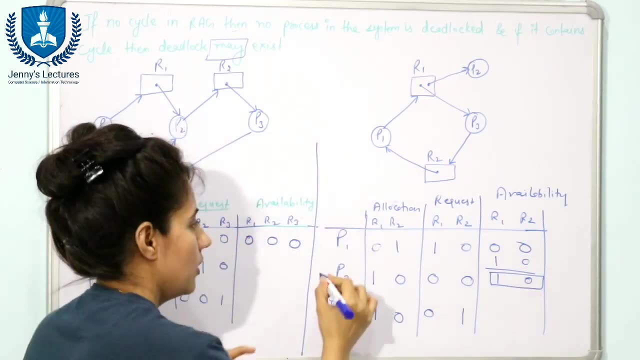 1. 0.. Now availability is 0. 0.. It release 1. 0.. Now total would be 0. And 1. Now available resources are 1. 0.. Now P2 got completed. 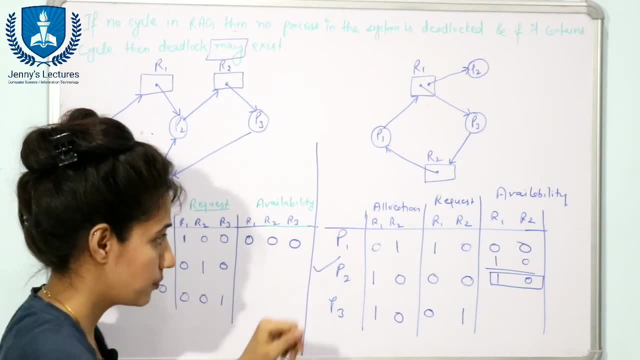 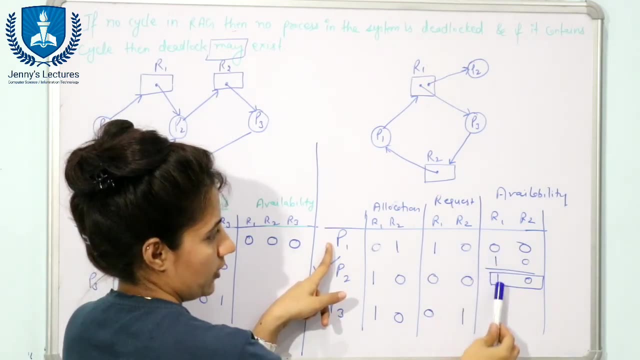 Now check out Which P1. Or P3. You can. You can complete, You can fulfill which request With the help of This: 1. Of R1. And 0. Of R2.. 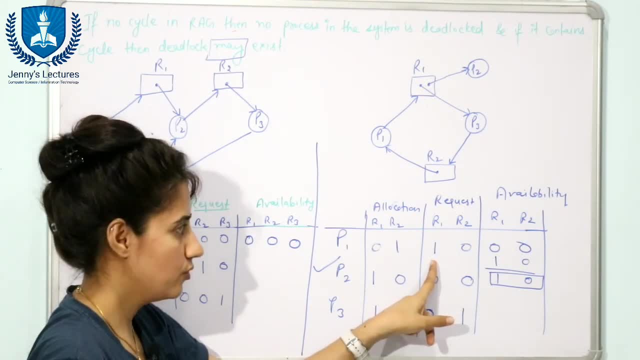 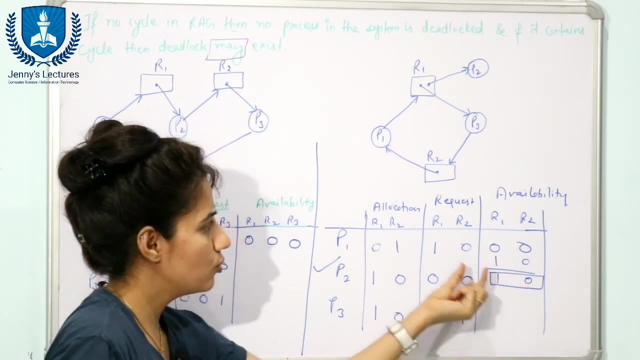 So we can fulfill this request Because P1. Only requirement: The requirement of P1 is 1 instance of R2.. Fine, So you can allocate This resources to P1.. Fine, If you allocate These resources. 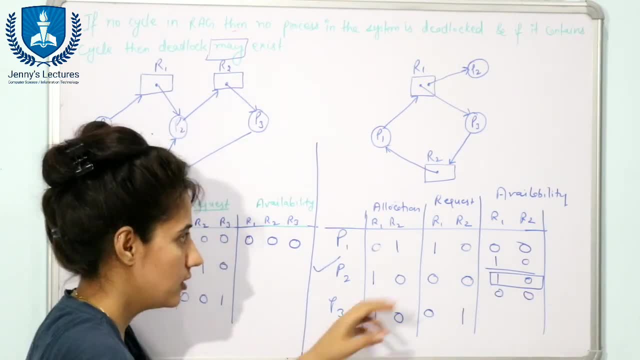 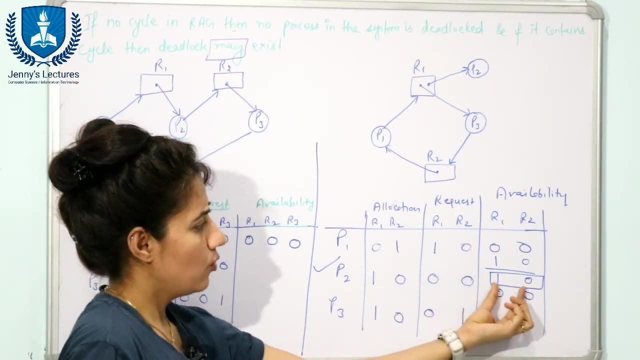 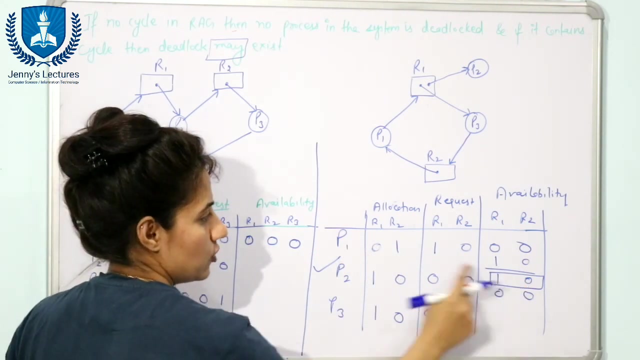 To P1.. Now availability is 0.. 0. Again, Because You have allocated this 1. To this P1. And 0.. After Allocating 1. And 0. The allocation: 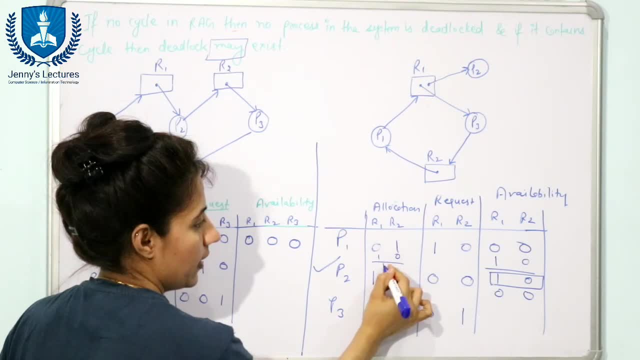 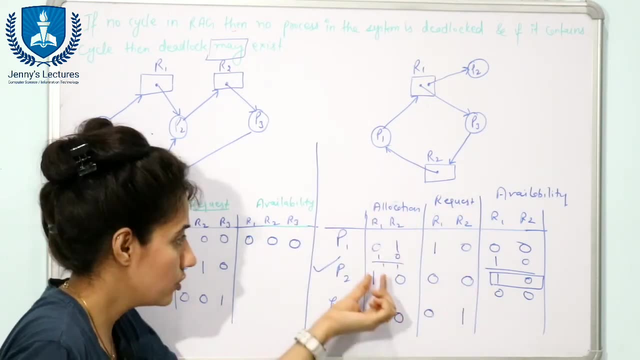 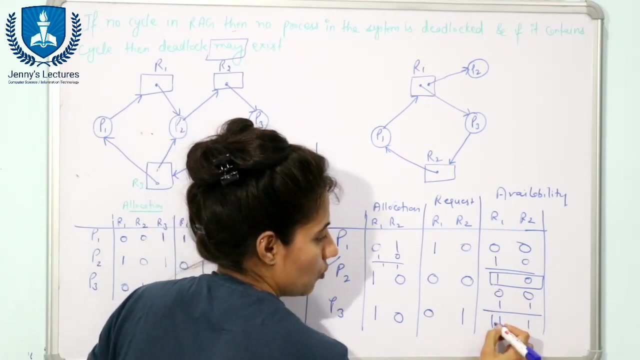 Matrix Of This P1. Bill Will Becomes 1. And 0.. Here You Will Allocate 1. And 0. The Total Would Be: And Request. 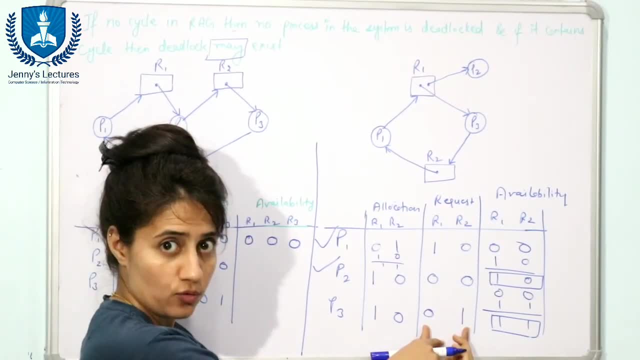 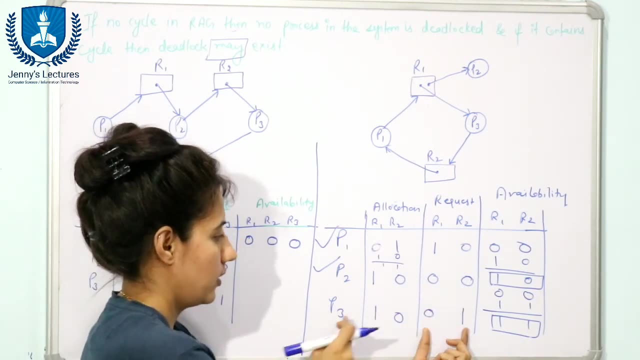 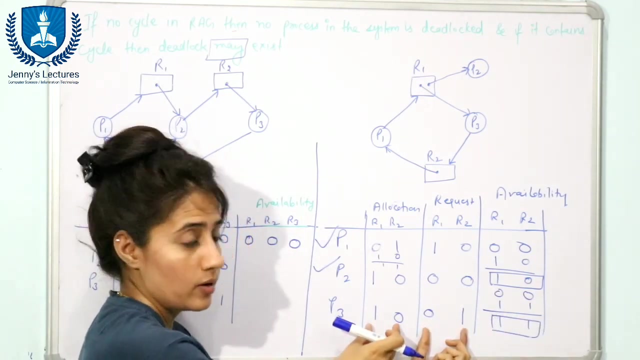 Of P3. Is Only 0. And 1. So Can We Fulfill This Request? Yes, We Can Fulfill This Request, So We Will Allocate. 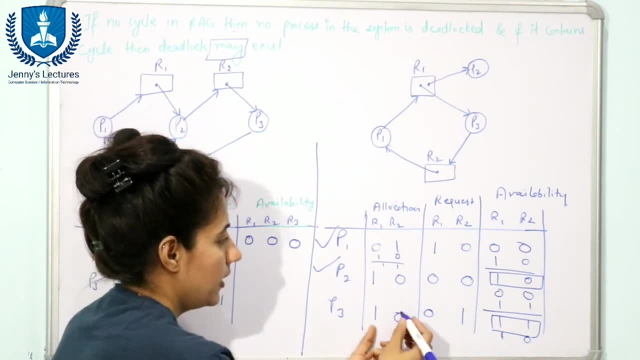 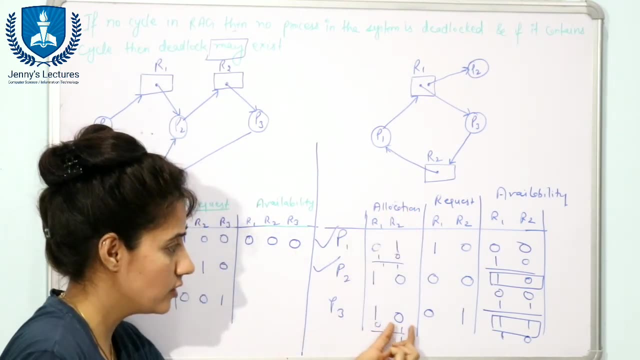 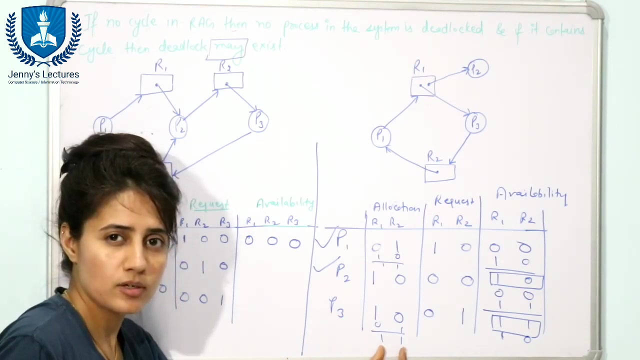 So It Doesn't Need This Becomes 0.. 1. 1. And 1. Because 1. It Already Hello, Already Allocated Are 1. 0.. 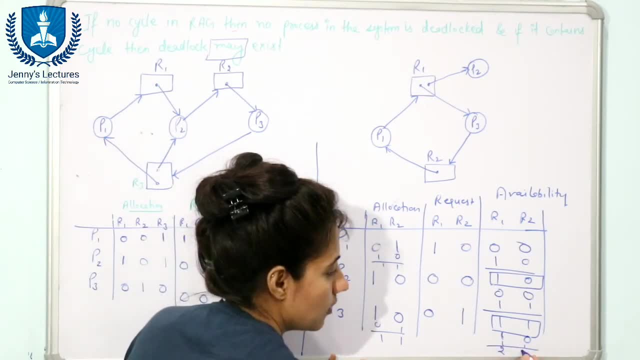 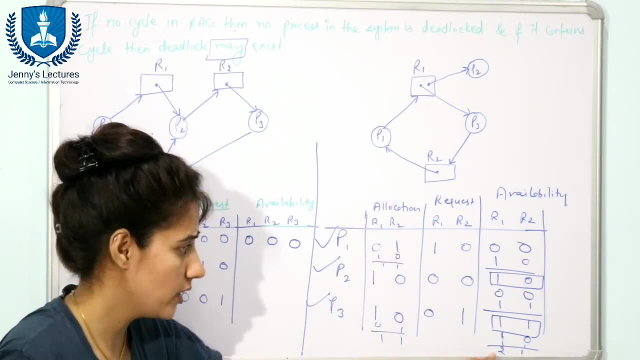 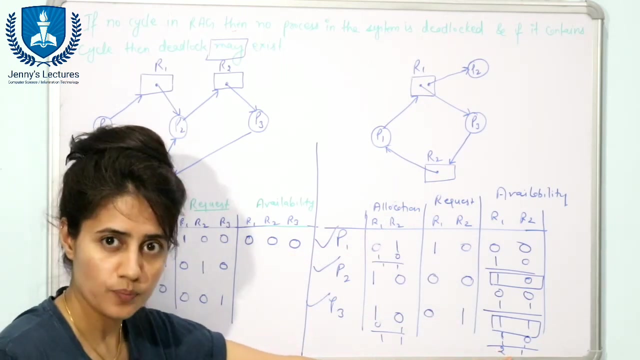 And 0.. 1. Is Again Allocated, So This Becomes 1. And 1.. So Can Request. This Is 0.. 1. And 1.. 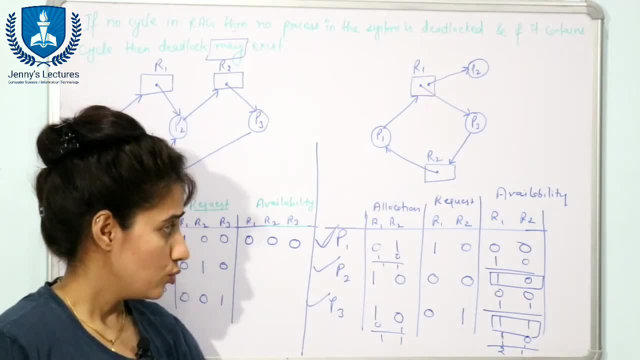 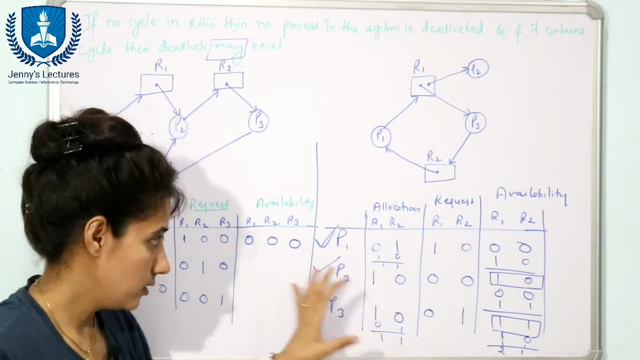 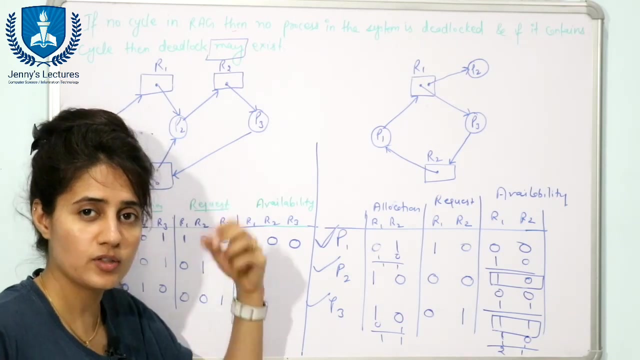 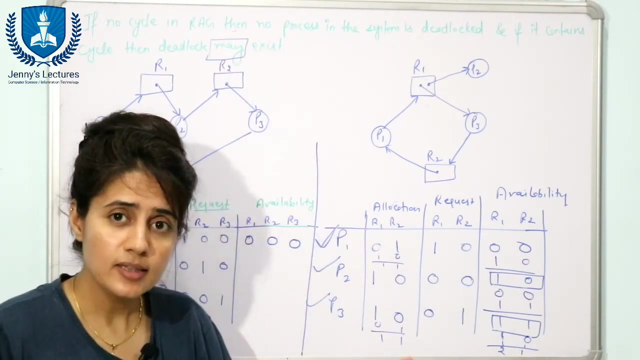 0.. 1.. Then This Is Really What We Can Allocate: 0.. 0.. You Can Yes Another This Can Allocate, To not see here the fund eyes. so if no cycle, then definitely no deadlock, but if cycle is there plus. 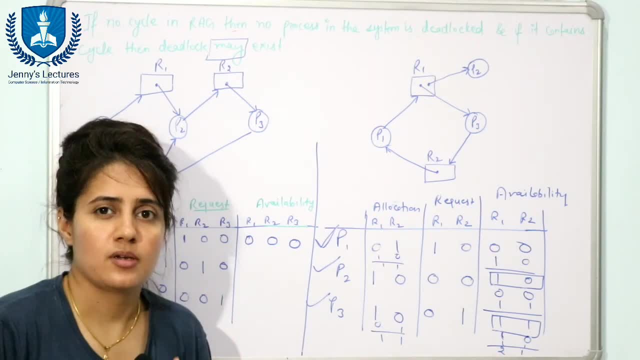 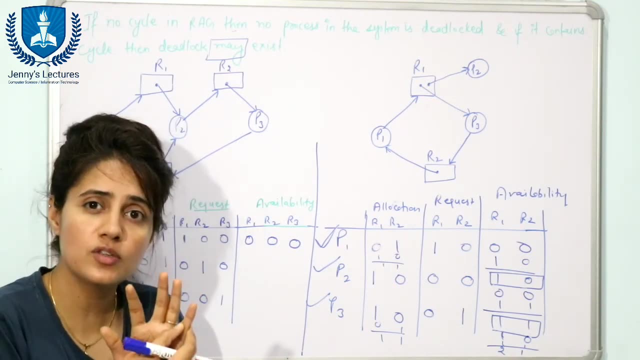 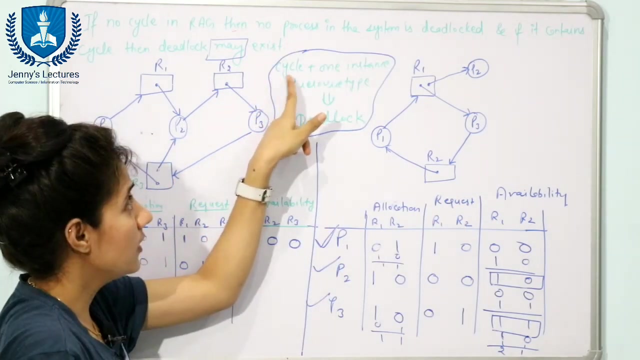 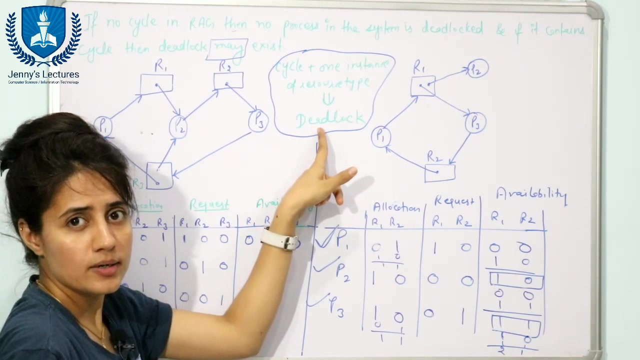 only one instance of the resource type is there. the resource type is having only one instance. cycle is there plus one instance of the resource type is there. it means definitely there would be deadlock cycle. if the resource allocation graph contains cycle plus only one instance of the resource type, okay, then there would be deadlock definitely. second case is if cycle exists plus. 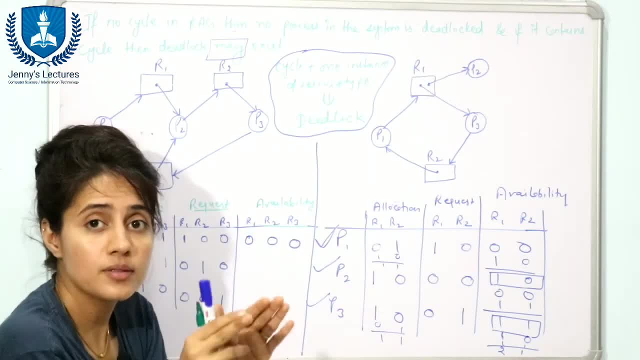 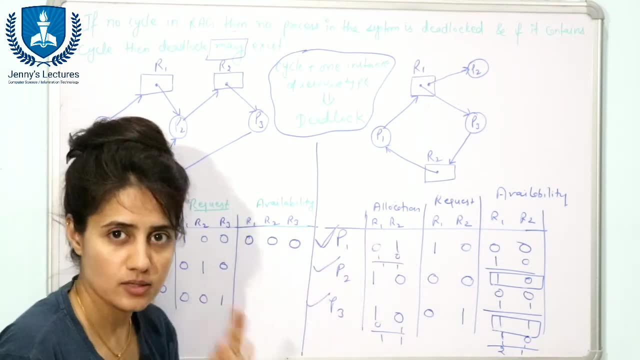 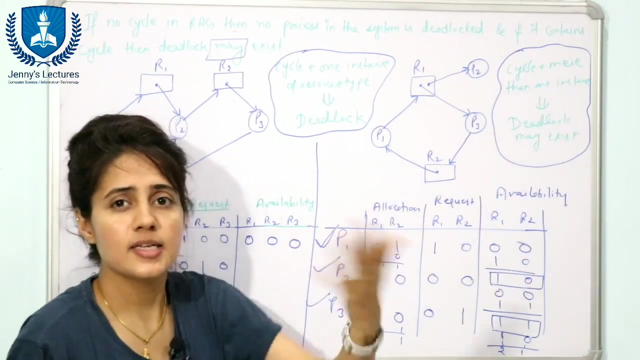 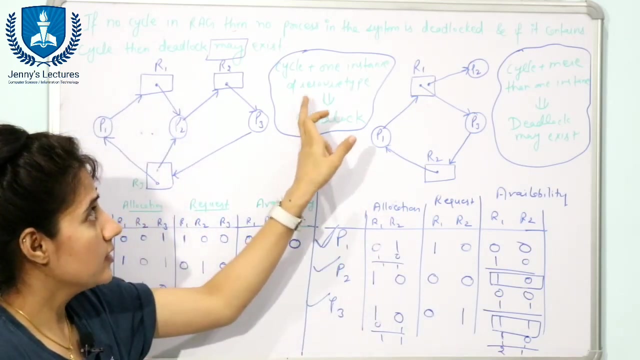 more than one instance of resource types are there, then deadlock may exist. you cannot say deadlock will exist, then deadlock may exist. and second case is: if rg contains cycle plus more than one instances of resource types are there, then deadlock may exist. fine, so in this case, in one instance, this existence of cycle is necessary. 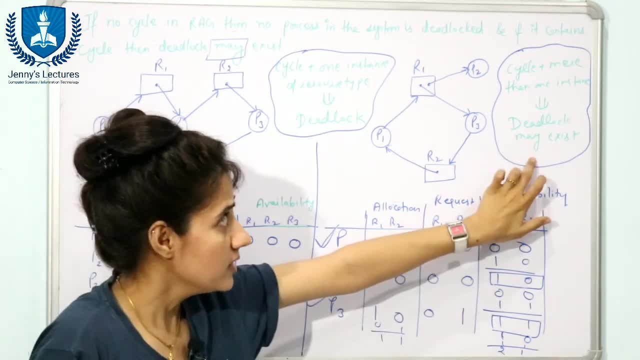 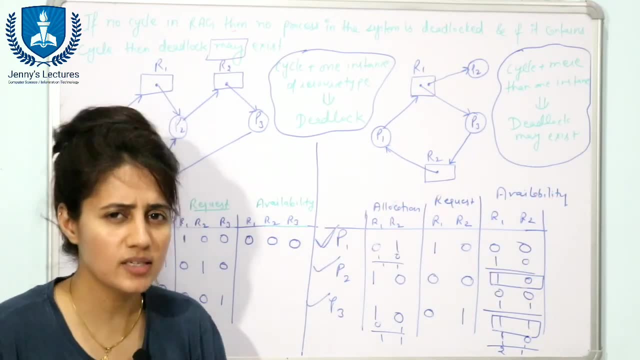 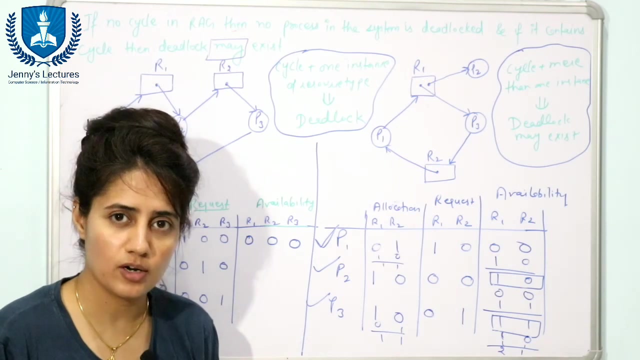 and sufficient condition for deadlock. but in this case, cycle plus cycle plus more than one instances are there, then existence of cycle is only necessary condition, not sufficient condition. and if no dead, no cycle is there, then there would be no deadlock. and the method? how to check from the 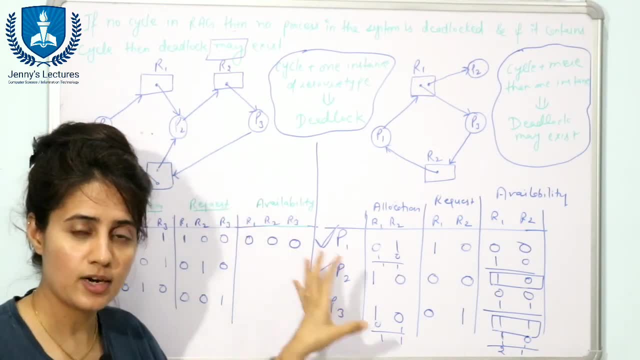 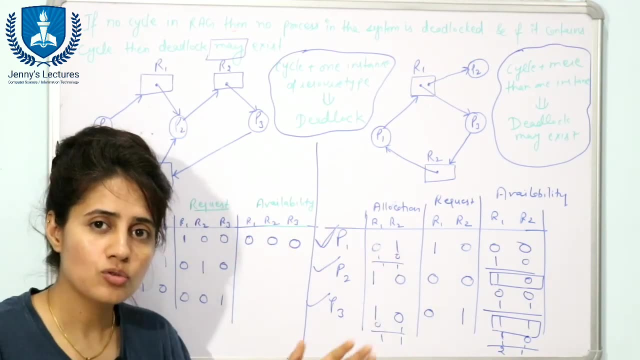 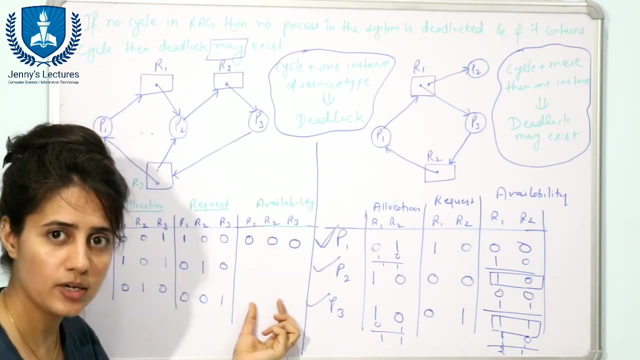 resource allocation graph that the system is in deadlock state or not, then either you can check manually. if small resource allocation graph is there, if complicated resource allocation graph is there, then you can follow this method: just draw a location matrix, request matrix and availability- current availability- and just check with that, with the help of that availability, and you fulfill the.